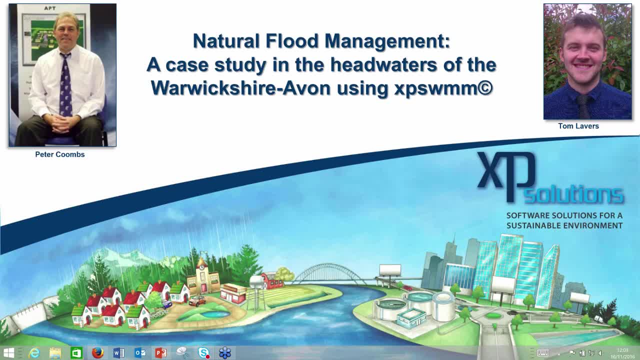 you'll have a little pop-up window. You can send in a message. We have a loop through Miller here as well. Thank you for looking at the messages for us, Ludi, And we'll endeavour to take questions and answer those at the end of the presentation. 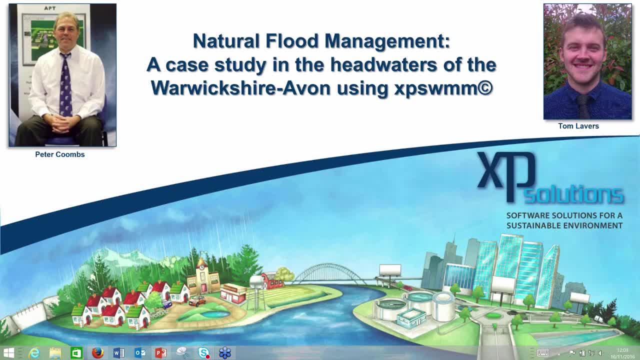 So, without further ado, I'll hand you over to Tom Great. Thank you, Peter, And thank you everyone watching who spared their lunch break for this particular webinar. Now, before we start, I'd like to make a few further acknowledgements to the project partners. 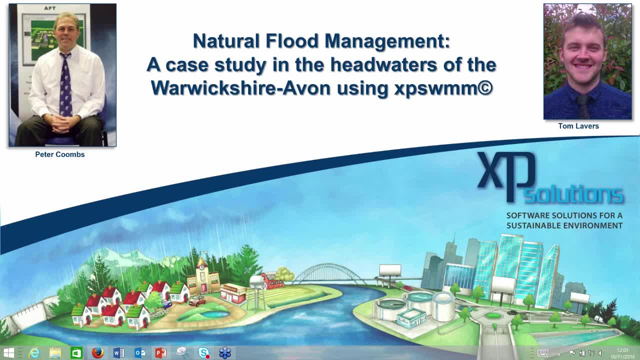 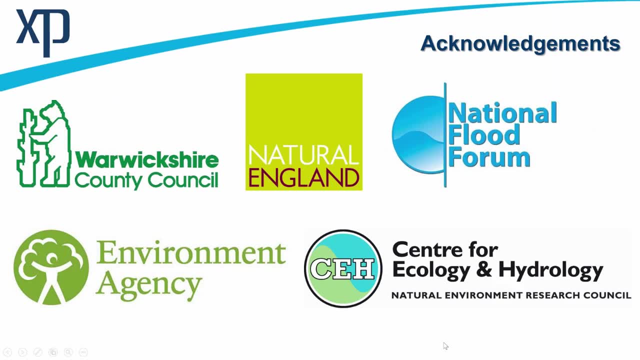 aside from the Centre for Agroecology, Water and Resilience and XP, This project has been in partnership with FCRM stakeholders funded by Warwickshire County Council as part of the English 7 and Y RFCC, who have been real drivers for this sort of catchment-based ethos. 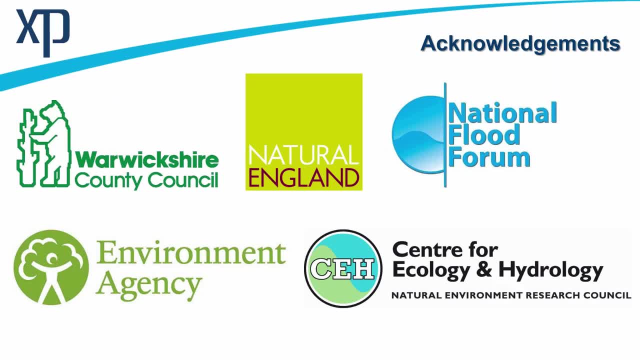 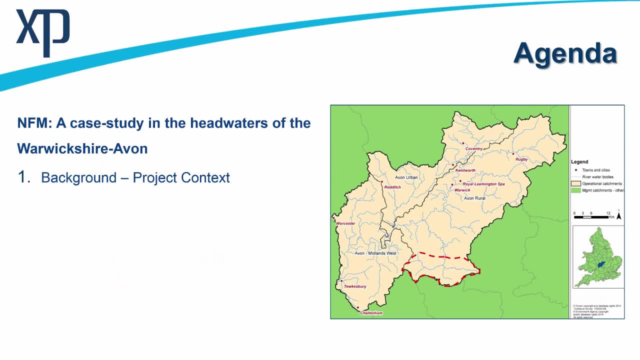 and who are also funding the Shrouds Rural Sudge Project and the good work Chris is doing at the District Council over there. Now for the agenda today. this webinar will discuss some of the methods, results and experiences as part of the first year of my PhD. 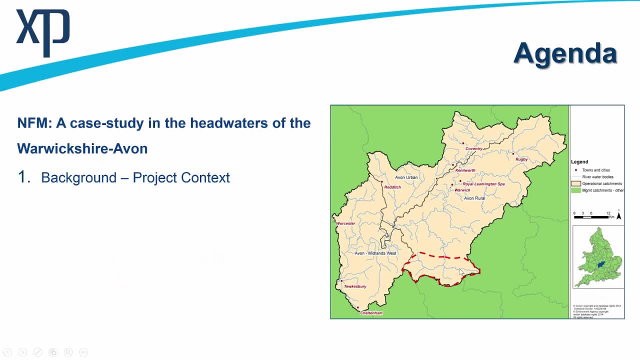 It'll be split into three dominant subsections. Firstly, I'll give you some sort of background project context defining natural flood management in regards to recent policy and practice applications over the few months and even days, Then discussing the specifics of my study area in regards to the issues NFM must address across the catchment. 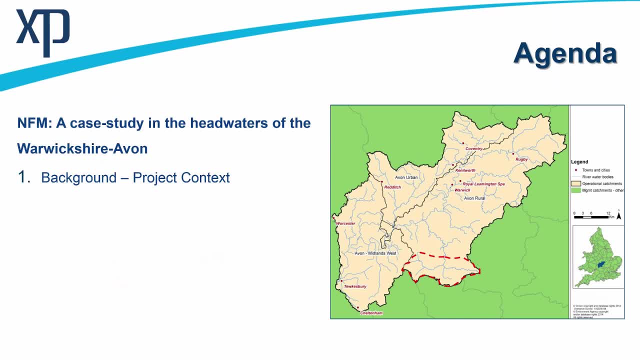 which you can see on the right hand side outlined in red, located in the headwaters of the Warwickshire Avon Rural Operational Catchment at the top of the Severn River Basin District, with the majority of the land use being intensely agricultural. I'll then touch upon how this research has tried to support meaningful engagement. 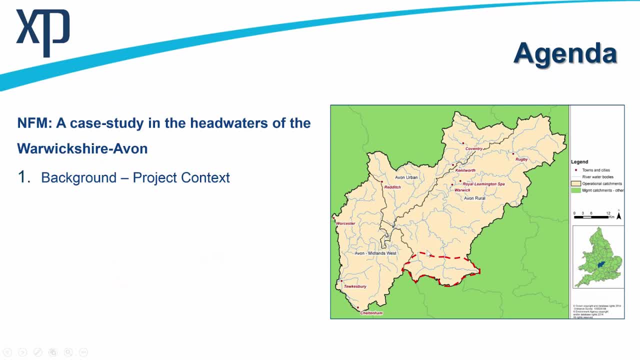 which, in my experience, has commonly come under criticism from past approaches and local communities that have felt local knowledge and concerns have not been considered when flood risk planning. Then I'll discuss the method applied to date and lessons from scoping and implementing natural flood management. 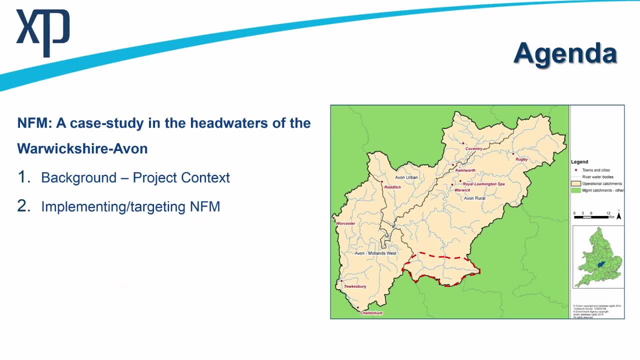 Now this will include, as Peter said, the preliminary results from the first year of this particular PhD, successes in the farming community at understanding the particular ethos of NFM and agricultural land drainage, alteration for flood alleviation And finally, I'll give you a little bit of background. 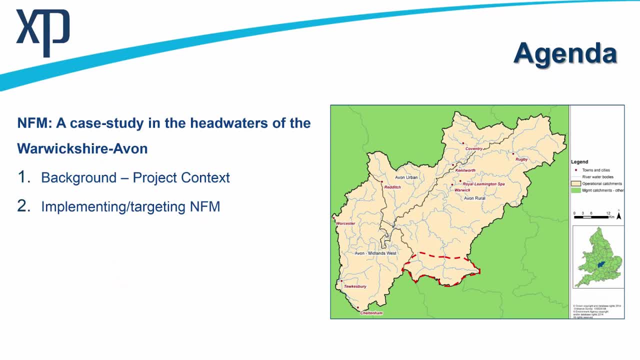 I'll talk about some of the negatives associated with funding an NFM catchment based approach, considering the current silos of funding and how the gaps in research can be filled with the overall aim of this PhD, which is to really value a meso-catchment scale NFM scheme, and the importance of using appropriate modeling software. 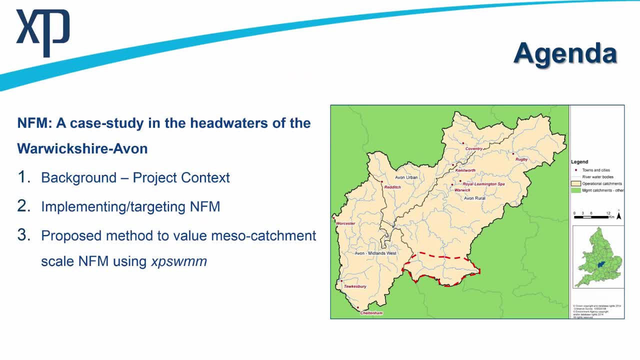 Now I'll discuss how the research aims to address some of these funding issues, using the study area and the XP-SWMM software to understand catchment systems hydraulically and hydrologically, And how we can go about appraising and targeting meso-scale NFM for different rainfall scenarios. 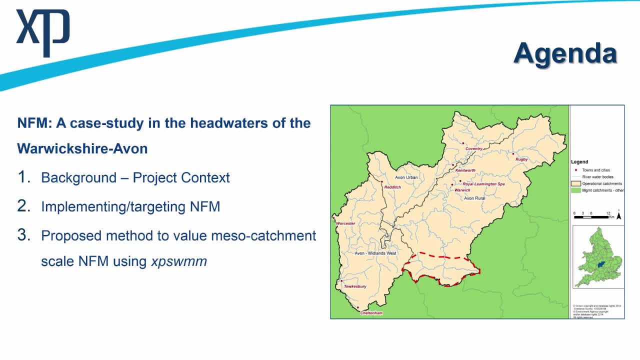 Now some considerable headway has been made with the array of projects since the multi-objective pilot investigations back in the year 2000.. But I hope you can see the need for more investment in time and understanding of this particular field. It's also worth noting the modeling is, as Peter said, in infancy and it's insensitive. 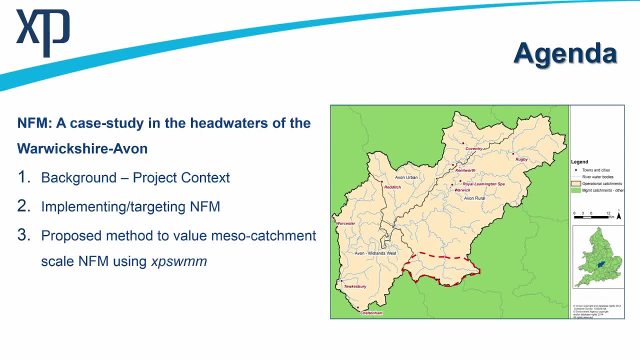 However, I hope to take you through a step-by-step methodological guide. I look forward to receiving any questions and comments, And I also hope that this webinar can act as a multidisciplinary guide to all backgrounds- not just modelers- interested in working with natural processes on a catchment-based approach. 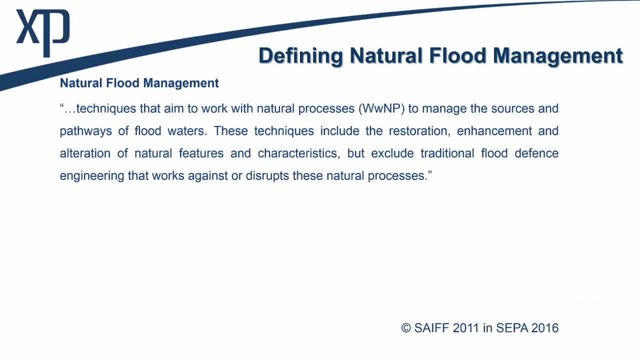 Now I've taken a slight Scottish leaning with my interpretation of natural flood management and the NFM constitutes techniques that aim to work with natural processes to manage the sources and pathways of floodwaters. These techniques include the restoration, enhancement and alteration of natural features and characteristics. 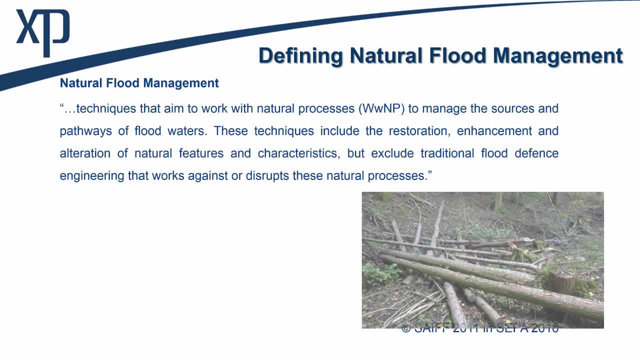 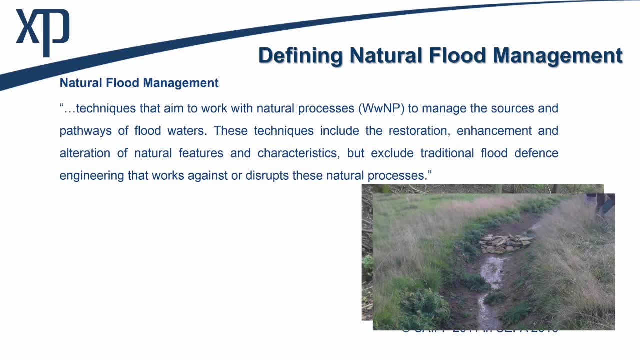 examples of which include: in-channel mechanisms to attenuate floodwaters, such as large woody debris dams. This is an example from the Stroud project. Alteration of the drainage pathways with other damming materials, such as this stone used in the Honeydale Farm project. 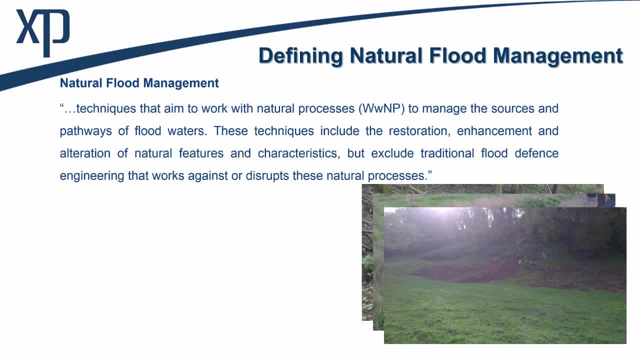 There are also floodplain features such as bunds acting as sediment traps for intercepting pluvial flow, And this image is also taken from the Stroud project. Now, NFM does exclude traditional flood defense engineering that works against or disrupts these natural processes. 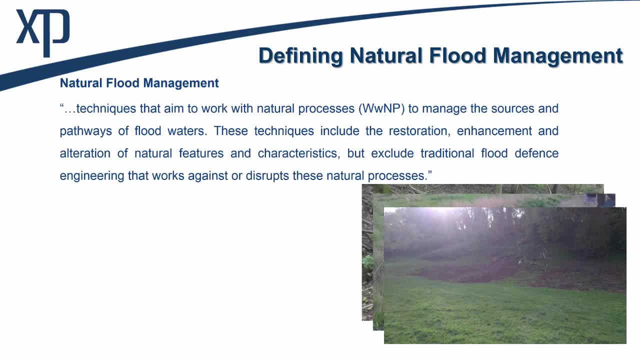 Now by traditional flood defense engineering. I'm referring to what has historically been the means of managing flood flows, conveying them in hard-engineered structures away from people and properties downstream at higher discharge rates. An example of this is, ironically, the view from my office. 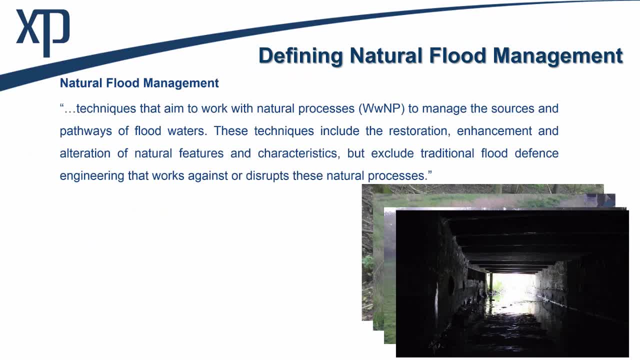 No, I don't sit in a culvert, but I am based in Coventry and the heavily modified River Sherbourne is culverted under the majority of the city centre with some exposed points for trolley tipping. Now, as I'm sure you're aware, the concerns with this historical method. 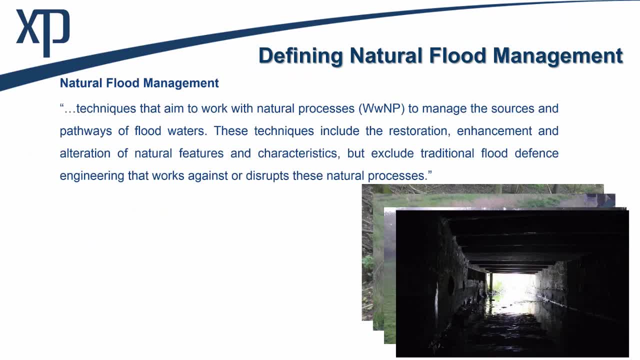 is the limits in capacity, and those who have worked in such retrofitting will know it can often be extremely costly enlarging traditional drainage capacities, especially with the influence of reviewed climate change allowances. Now, when I started this particular research, I commonly came across many other researchers. 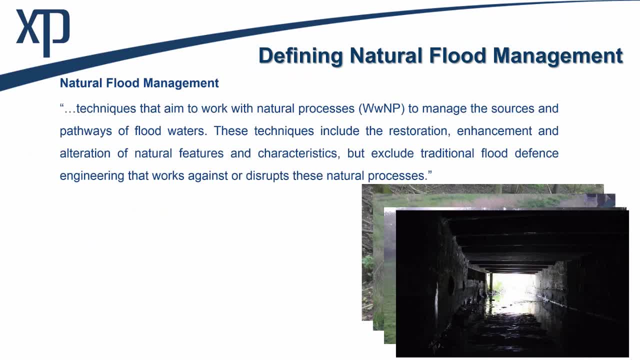 that said, NFM is reinventing the wheel and that these sorts of approaches have existed for years, including rural suds, permaculture, farmer retention, etc. Now I would agree. the components within NFM are techniques that have been employed for years. 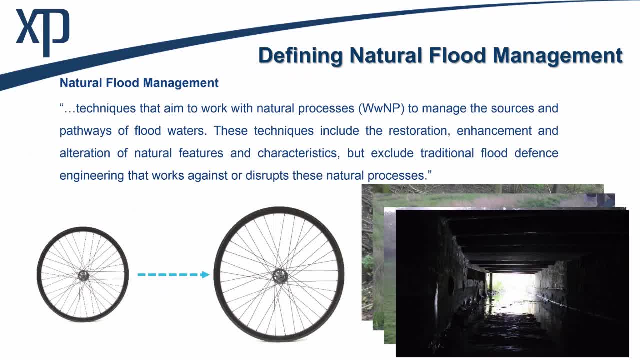 but as an ethos. it's not just reinventing the wheel, but enlarging it. And that's where the real challenge comes: understanding how these measures interact holistically when upscaled, which brings me to my next point: the significance of scale. 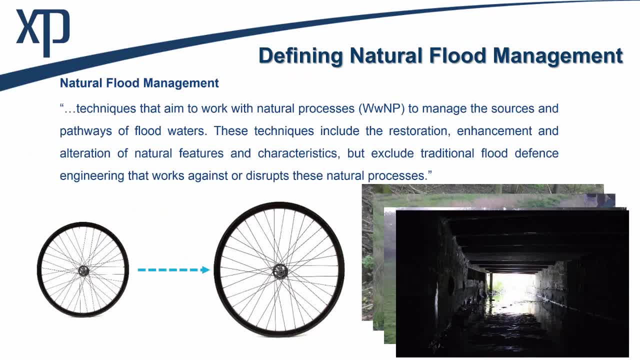 Now my fluvial catchment is 187 kilometres squared, with a variety of different sources and pathways of floodwaters which impact different receptors at different times. Previous computational methods and data sources have found this a challenging task, with resolution and reliability being a key issue. 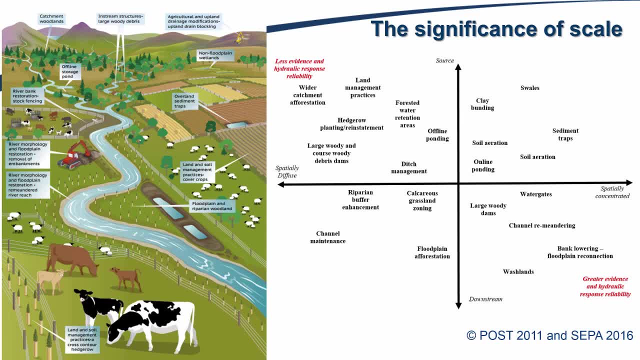 But advances over the last 40 years or so have allowed us to obtain a better understanding of catchment systems. However, the derivation of relationships between the rainfall over a catchment area and the resulting fluvial flow is a fundamental problem for hydrologists at this sort of scale. 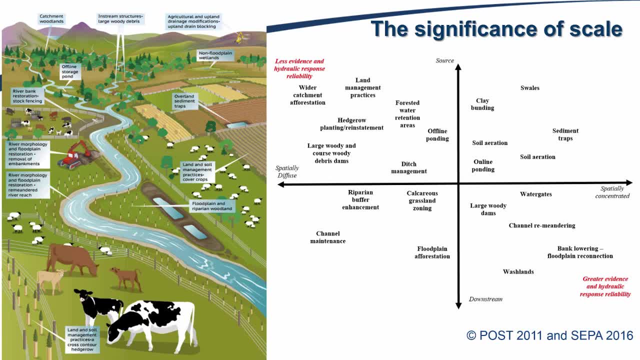 that many of you watching will be aware of Now. on the MISO scale, XP-SWIM's ability to illustrate spacemodic rainfall and differing surface influences, such as your soil types, geology, land cover and, significantly, the spatially heterogeneous antiseptic. 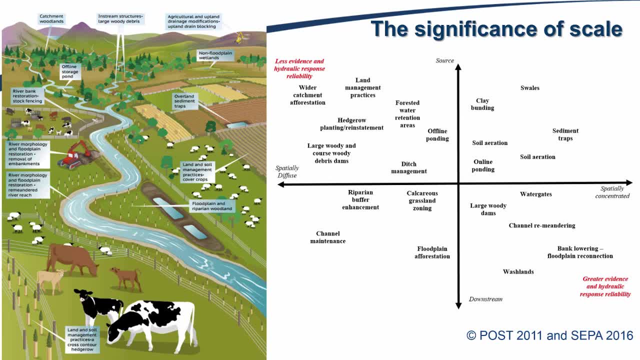 and pedological conditions that affect infiltration rates and overland flow types is critical. Now, as some of you may recognise on the left, this is an image view of different NFM features in different locations across a catchment from the SEPA Natural Flood Management Handbook. 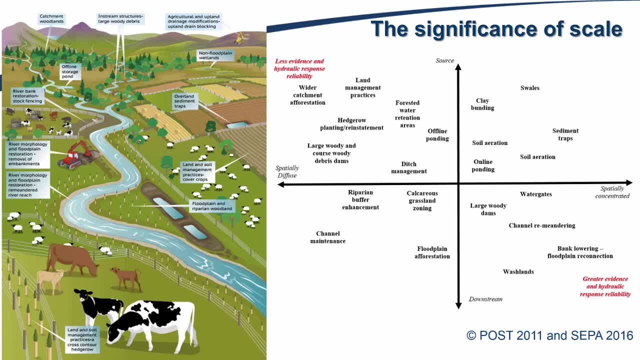 Now, as you can see from the matrix on the right-hand side, adapted from Thornetown in 2007,, is that these measures interact at different scales and locations. This matrix indicates the different suggestions. I've mapped across the catchment, but I'll go into more detail on that later. 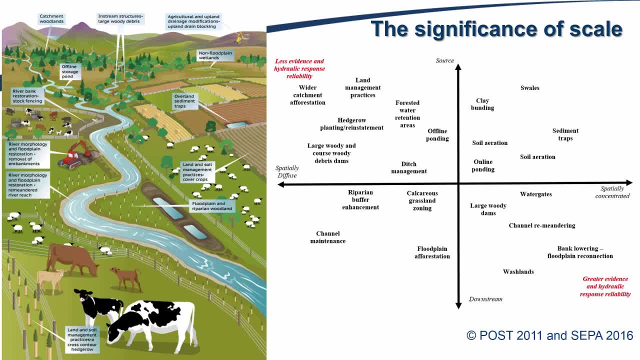 But, as you can see, measures at the source, such as wider catchment, afforestation and runoff attenuation features, as coined by the great work in Belford, are at a spatially diffused scale As we work our way down the catchment to points of floodplain reconnection. 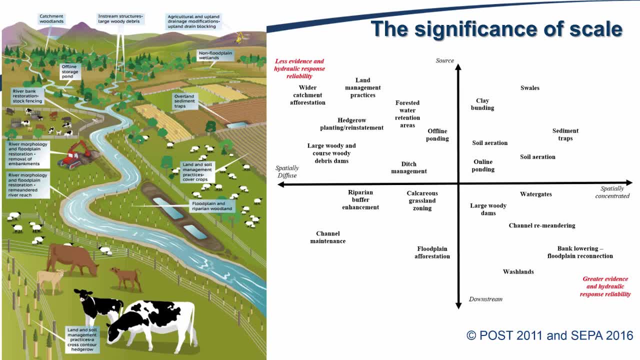 you know you're looking at bank lowering here and washlands. it becomes clear that conventional modelling techniques of the 1D environment are more reliable in determining the effectiveness of these schemes at retaining flow. This is likely due to the spatially concentrated nature of the scheme's nature. 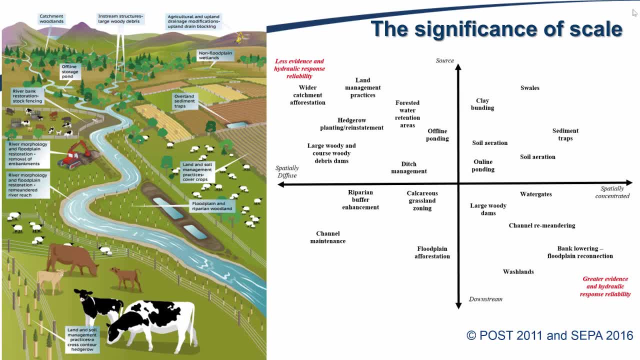 which can provide sort of meter cube storage values per area of retention. However, what research has found to date is that these downstream measures need to interact with the upstream in order to attenuate flows more successfully. We're looking at an aggregation effect. Of course, these are dependent on your individual catchment context you're working with. 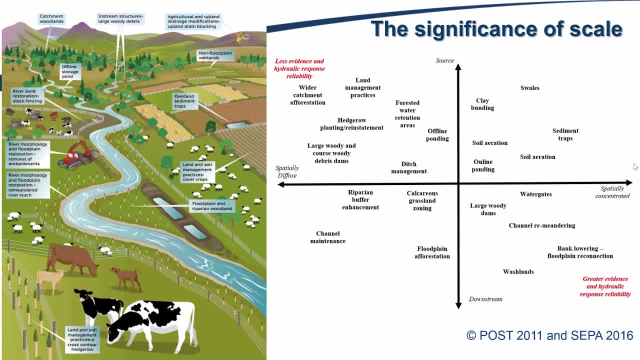 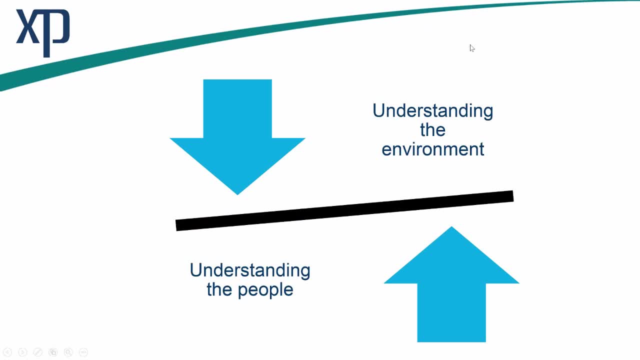 and, more importantly, the areas of risk you're trying to alleviate, Because really what we're trying to do is integrate flood risk management through a more rounded means. Apologies for the slight woolly-headed academic bit, but we're trying to understand the balance between people and processes. 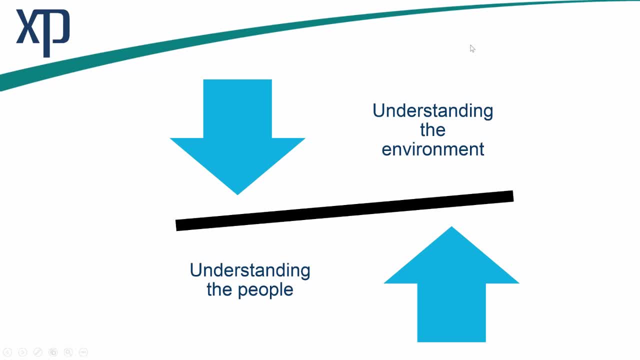 How do the people, such as farmers, impact the catchment's flood propagation, as well as how the flooding impacts the properties, businesses and farming communities themselves. Now, in terms of practicalities, the application of these schemes and what it means on the ground is key. 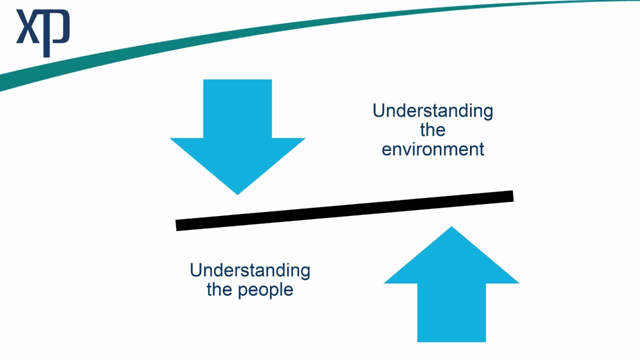 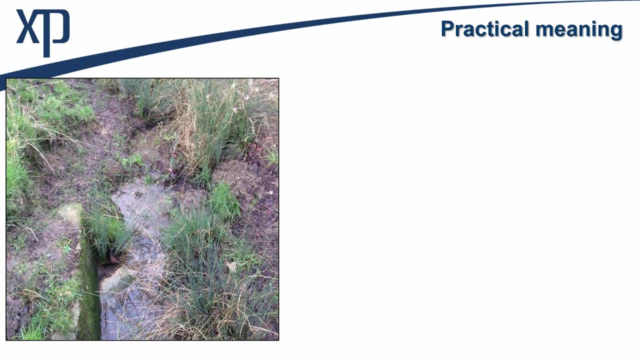 In principle, past drainage techniques across agricultural catchments, as is my patch during wartime intensification- have been based on great levels of underdrainage, as shown on the left, commonly with stock grazing such as sheep, and leading to improved grasslands of clays. 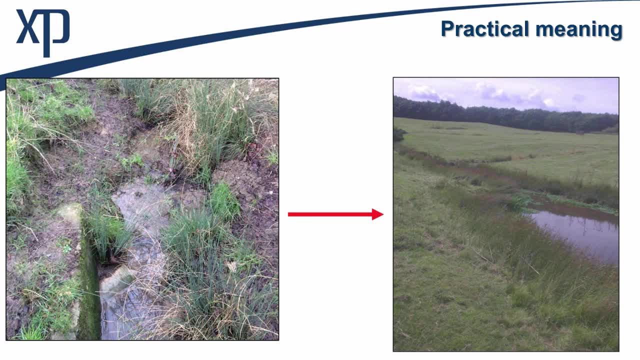 Now we need to consider how we can review pipe-based schemes, such as your mole ploughing to areas of semi-permeable retention, like the ponding area on the right Now. both these images were taken in different parts of the catchment. 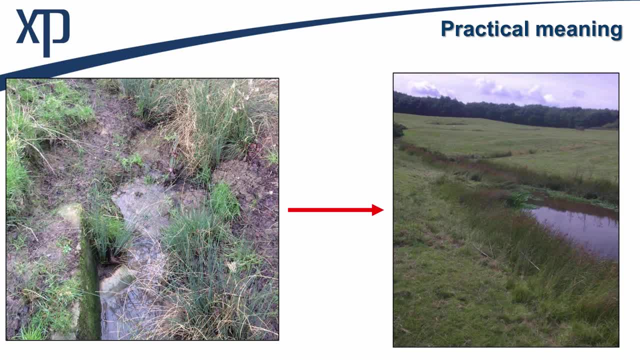 Now, whilst I won't mention the landowners by name, it is clear that local champions can make a real difference in supporting best practice when it comes to altering farm drainage And, as I said previously, what I'm really trying to do is protect properties and businesses. 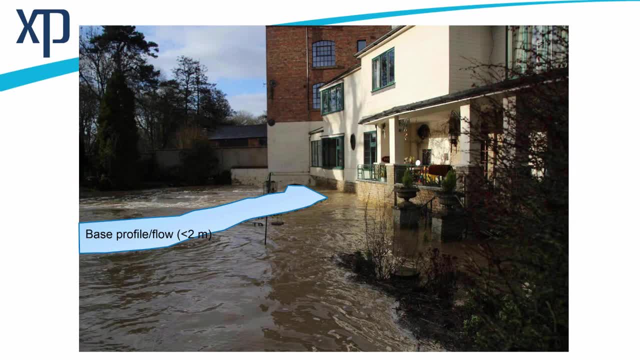 Now this particular event internally flooded this property 30 minutes later. It is located at the downstream extent of the study site with approximately six hours of warning, and required the carpet to be quickly lifted and belongings moved upstairs Once ingress occurred. it took the owner weeks of drying and clearing. 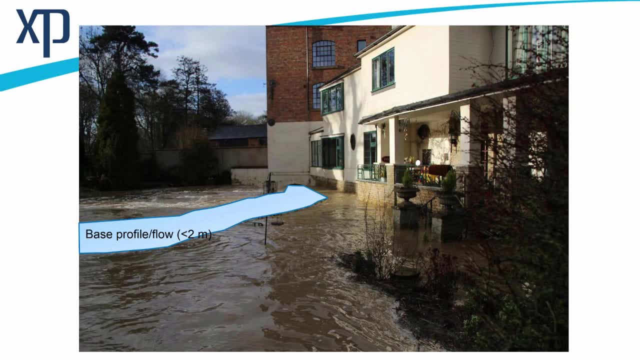 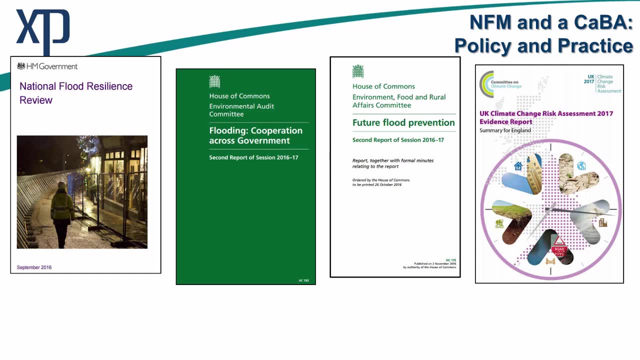 before being able to make the downstairs of the home livable again. Of course, investment decisions and agendas are driven by policy and practice which, over the past months and even days, have been very much pushing NFM and catchment-based approaches. Please see some referenced key documents. 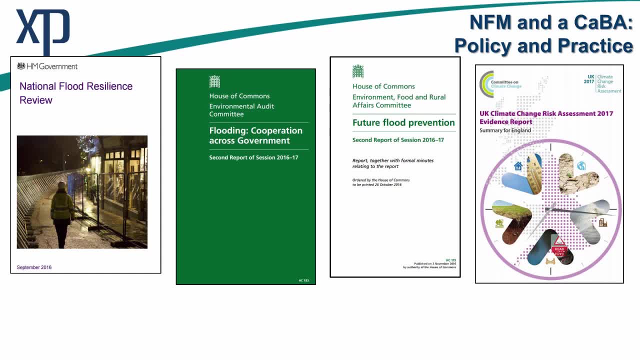 Now, most recently, the EFRA committee report highlighted the importance of developing these catchment-based plans to manage flooding at the large scale, technically being in excess of 100 kilometres squared. Now, in defence of those agencies involved in managing flooding, I think it's worth noting that this sort of approach 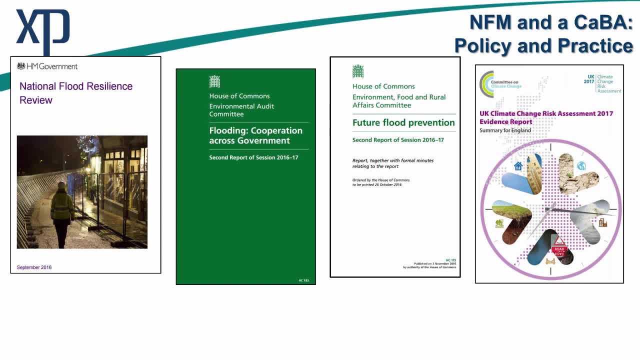 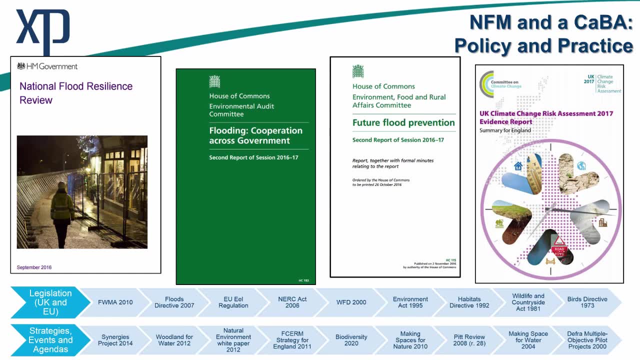 has been in the pipeline for quite some time, as we've been going with the flow, as it were- And this is in reference to the diagram at the bottom of the page and to many of you watching who will have either completed or are familiar. 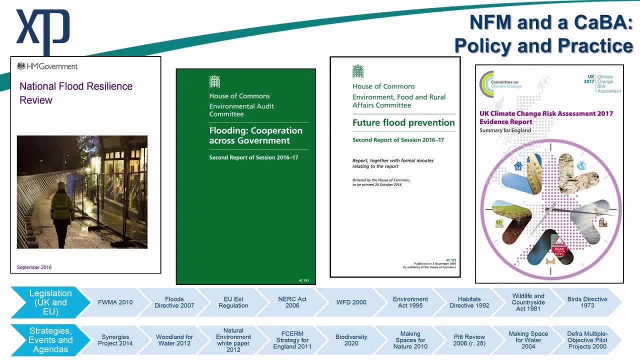 with lots of similar case studies occurring nationally that have been ongoing for some time, trying to better understand the science behind the sort of largely theoretical field. Now it is clear end of pipe and last line of defence. approaches are unsustainable, as shown in the winter 15-16 events. 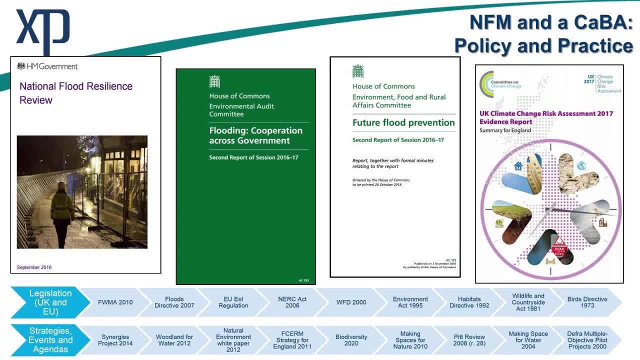 Since then, considerable investment from DEFRA and EA, both financial resources and expertise, such as the Working with Natural Processes Group, publications with the EA and supporting consultants such as JBA and others, have supported this ongoing knowledge-sharing exercise that I hope today can be for you all too. 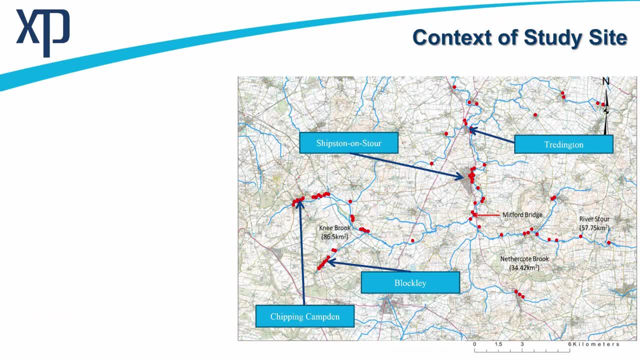 Now back to my study site. As you can see from the right, the headwater extent is made of three dominant feeds that flow south to north. You have the Knee Brook, Stour and Nethercote Brook. Collectively, it's 187 kilometres squared to the downstream node. 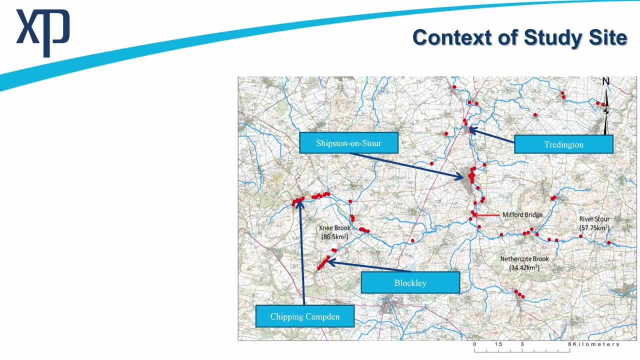 the Shipslawn Stour River Gauge. In terms of issues, there is a high flood frequency that leads to internal flooding of properties and businesses indicated by these red blobs, exception being the July 2007 event that flooded in excess of 180 properties across the catchment. 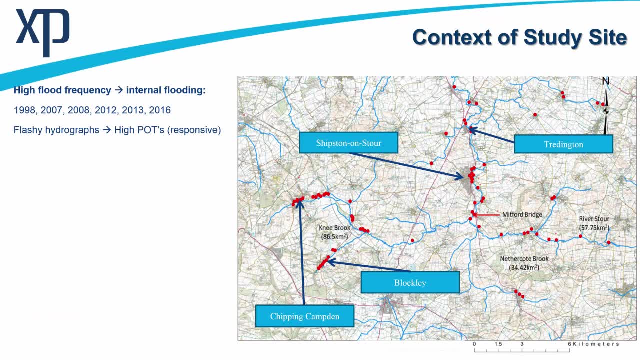 and, most recently, the March 2016 event that flooded four, And what we have are muddy flows, flashy hydrographs and high peak over thresholds recorded from the only National River Flow archive gauge, leaving little warning time and a bit of an indication of some synchronised flows. 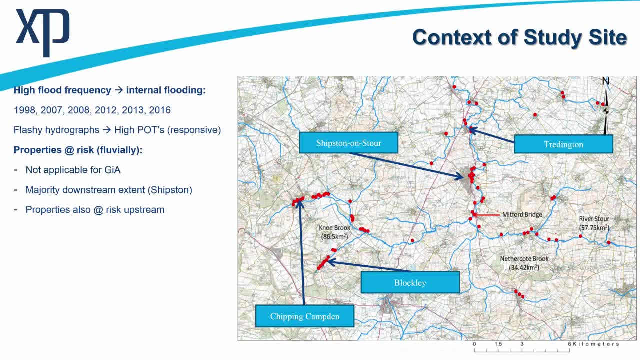 Now, in regards to the risks due to the spatial nature of the properties, none have been able to qualify for granting aid due to the level of costs associated with localised engineered schemes. Furthermore, pre-2012, on the involvement of the DEFRA Pathfinder project. 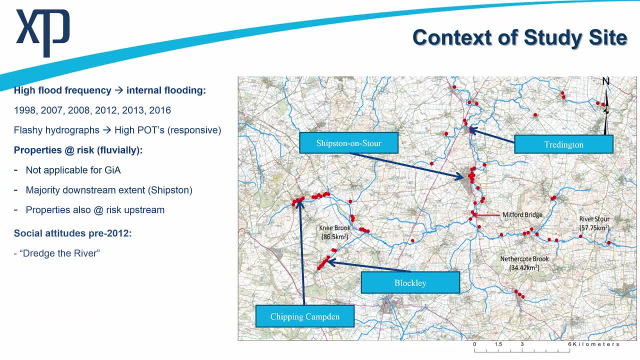 spearheaded by the National Flood Forum. many communities believed desilting bridge arches and dredging rivers was the only means of addressing peak flows. Since then, expert advice has highlighted the short-term issues with desilting river profiles downstream if continued silt contributes upstream. 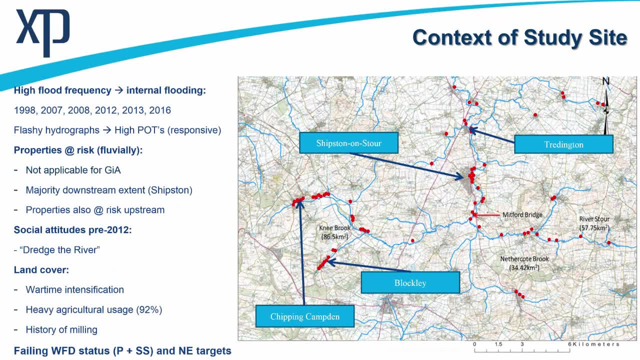 Now on the topic of silt, the catchment is failing WFD status due to sediment-attached phosphate issues impacting macrophytes and phytopenthos populations. This is recognised to be due to the dominant diffuse source from agricultural land use. 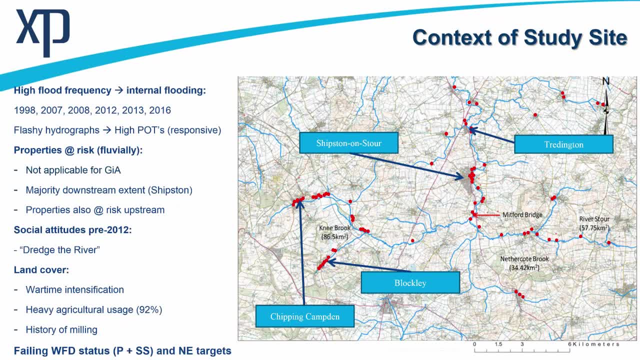 with many Natural England targets for stewardship in the agricultural environment- previously entry-level stewardship, high-level stewardship that's now transferring to countryside stewardship- that have failed to be met, many of which indicate areas for alteration for flood alleviation purposes and planting for water quality improvement. 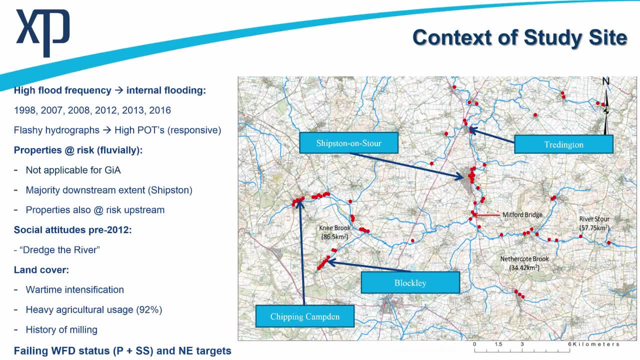 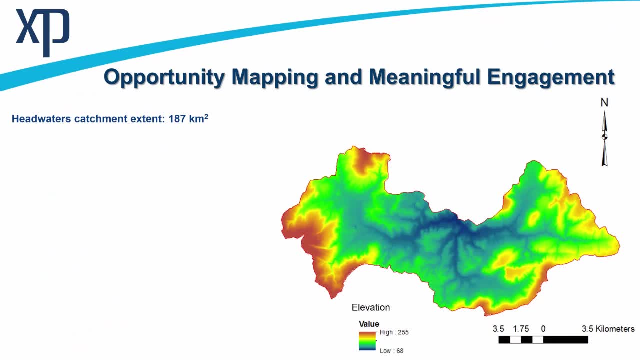 Now, hopefully, you can see that any scheme has to be holistic in its approach that can work for all stakeholders across the catchment. Now for the first task of my PhD. it was important to characterise the catchment area and understand where it might be possible. 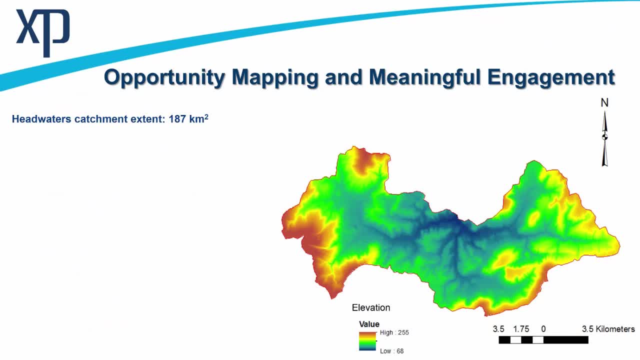 to locate features that can slow, store and filter flow. This slide will take you through this process step-by-step, to inform how data and qualitative input can inform a bit of a rounded understanding of the catchment Now. firstly, it was important to understand 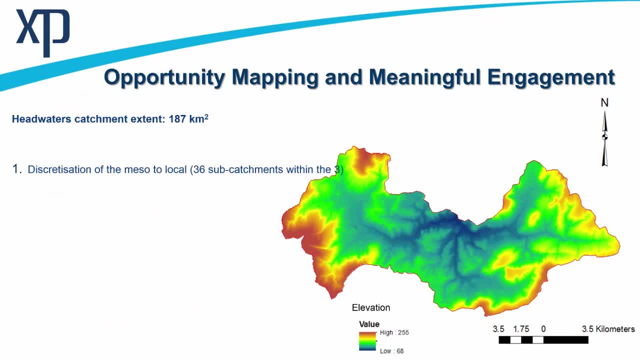 the scale of contributions. Therefore, discretisation of the three dominant tributaries into the 36 local-scale sub-catchments allowed for a more manageable task. This is also a time-saving exercise when relaying mapped outputs to the modelling stage when scenario assessing the timing of hydrographs. 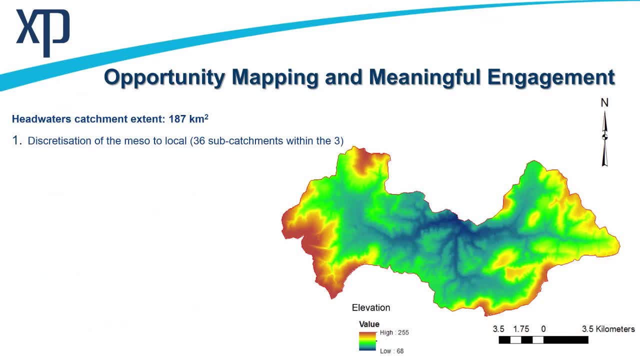 from sub-catchments, as available to do in XP-SWMM. It was then important to use GIS hydrology tools to do this, including watershed delineation in the ArcMap 10.4 software, building a reliable DTM from verifying elevation. 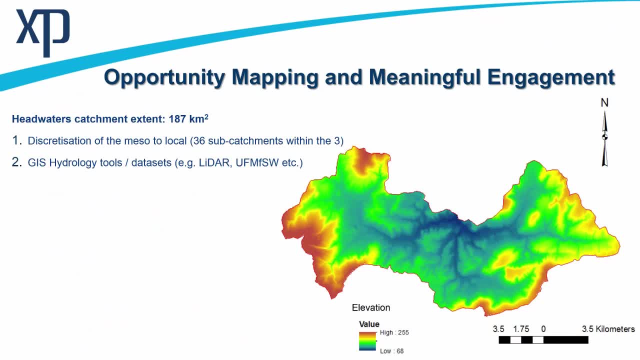 and LiDAR coverage, identifying key runoff pathways in conjunction with updated floodmats for surface water and fluvial flood extents where evulsion occurs. The LiDAR was made freely available from the Environment Agency Geostore site. an existing model. updated floodmats for surface water. 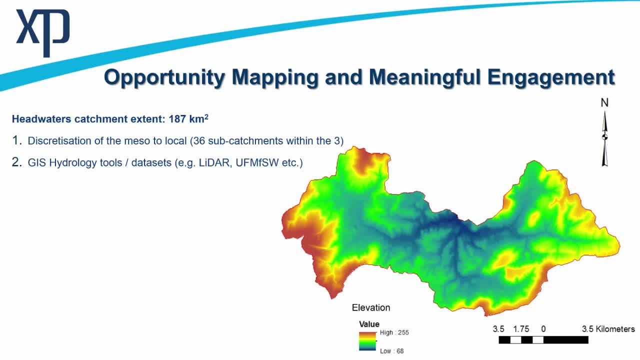 and fluvial flood extents available from the LLFA and EA. This was supported by hydrology of soil type data known as HOST geology, and Land Cover Map 2007 data to indicate infiltration rates, surface roughness patterns that all influence the existing flow pathways. 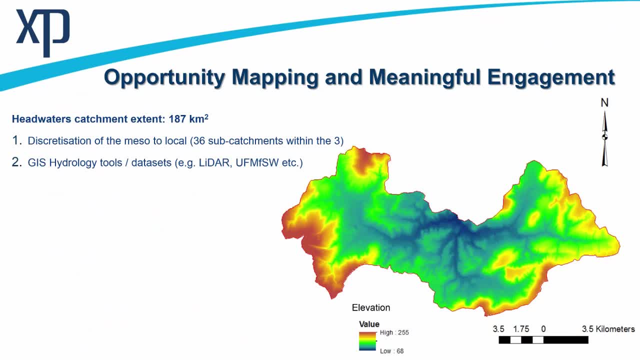 and types of NFM features that could be located. Furthermore, identifying locations of previous agricultural practice from historical pre-wartime intensification maps, such as previous areas of ponding, old land registry that indicates previous hedgerow boundaries. This all gives a temporal reference to RESTORE-T. 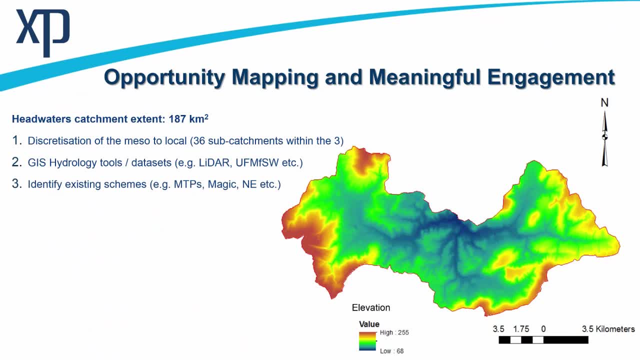 as well as an indication of possible measures in precise locations. From there, I was able to locate possible areas that could be suitable for NFM, such as points of ponding in the floodplain, as well as high Haltonian fluvial runoff pathways. 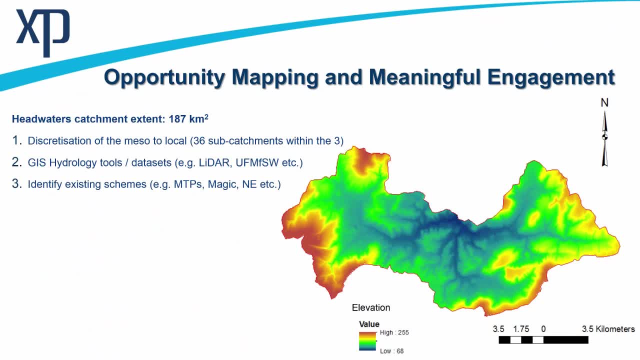 Then by overlaying existing schemes such as EA Median Term Plans and Natural England Stewardships available from DEFRA Magic Map. in conjunction with Tharma Consultation, I was able to understand what is planned for the catchment and what is currently being done to manage drainage. 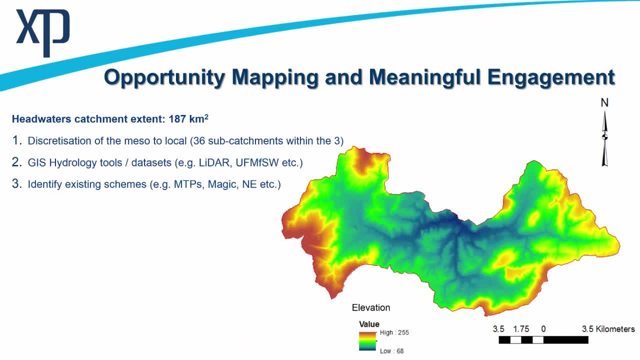 over farmland and wider environmental betterment schemes as part of the agri-environment agenda that can directly link with NFM. It was then vital for me to review many of the existing studies that have been conducted to understand best practice and specifically those in donor catchments. 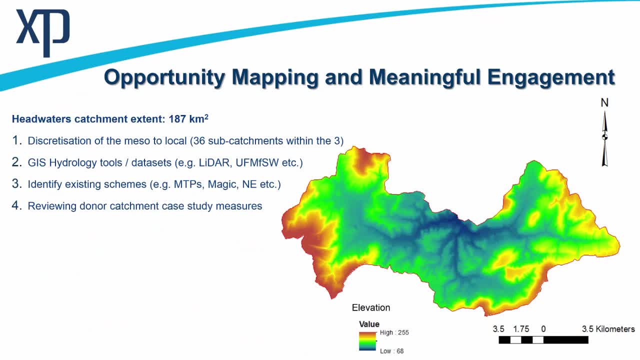 what sorts of measures have been employed, where and how. This supported the second and third steps by putting precise measures into particular locations across the catchment. These locations were reviewed, verified by extensive field walking undertaking, reconnaissance surveys and participatory mapping with the landowners and farmers. 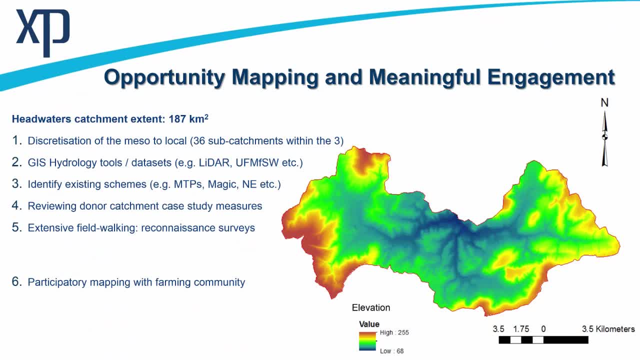 Now. the latter was initially undertaken due to the land being privately owned and requiring access permission. However, it became quickly apparent these stakeholders could provide local knowledge of their farmholding in regards to hydrological characteristics and influences of flood generation and propagation. Therefore, field walking photography. 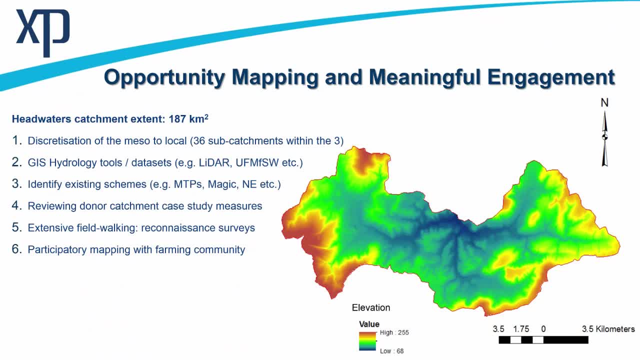 and basemaps from the previous steps allowed the farming community to comment on the locations of possible schemes, as well as commenting on what schemes could be more successful and mutually beneficial. Now, it's worth noting, a supportive local flood action group is essential in acting as gatekeepers. 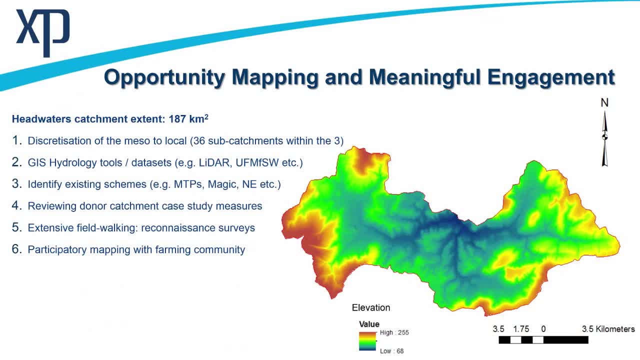 for this particular task. In my experience, external consultants and researchers have a different dynamic than local residents. Now this informed a map of opportunities, 318 in total located across this catchment And, as said previously, this current research stage is broadly conceptual. 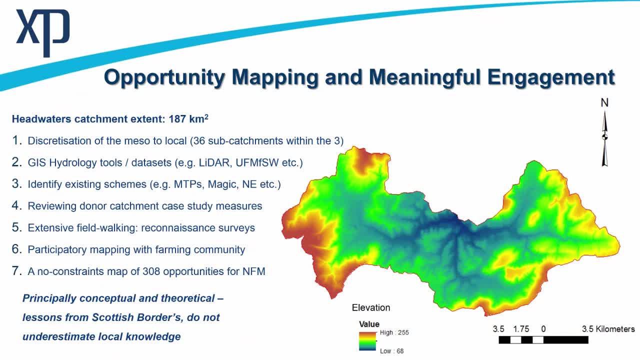 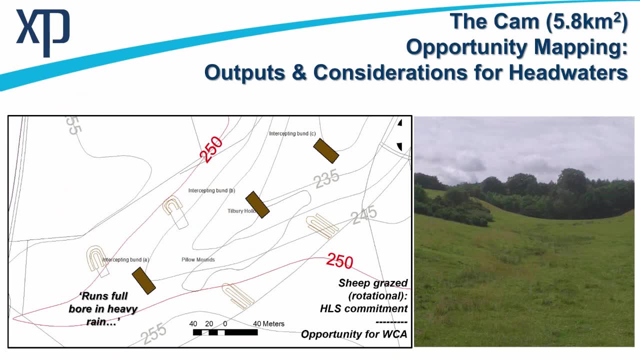 but, as Lessons from Scotland has found, we must not underestimate local knowledge. Now I'll quickly take you through an example: NFM opportunity in the CAM sub-catchment. This is in the headwaters of the Knee Brook On the left-hand side. 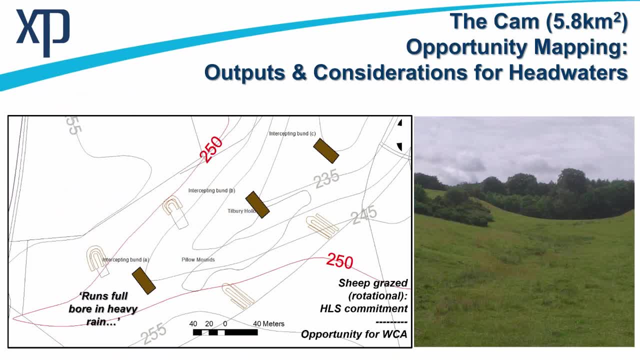 you can see the basemap of opportunities. This is a useful technique when discussing land area input and then commonly having some sort of particular field names that they then can relay to a master map. backdrop: The measures identified in this ephemeral stream, as shown by the picture taken on the right. 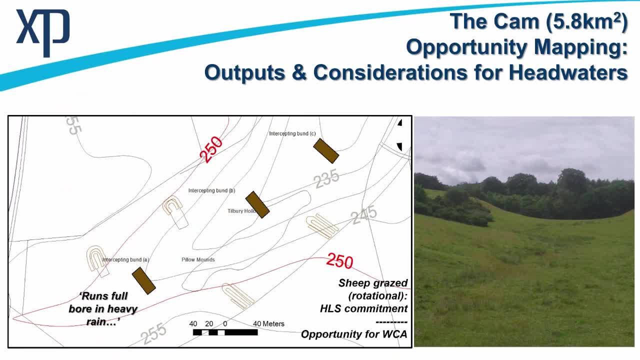 include clay bunds to act as runoff attenuation features. Now, the original locating of measures indicated this area as a possible space for wider catchment afforestation. However, the landowner was concerned how this would impact his high-level stewardship agreement with Natural England. 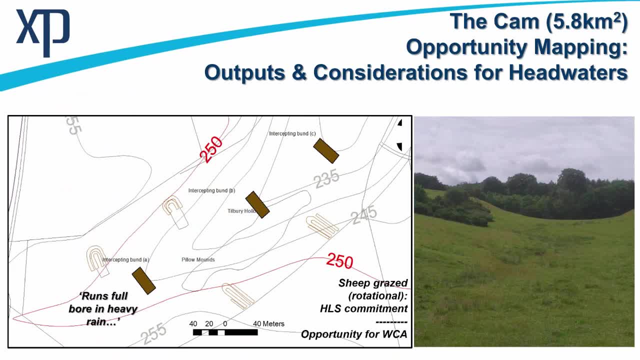 Therefore, using a pond calculating tool and an indication of water moving through an orifice outlet bund, it had the ability- each of these three bunds- to attenuate 35 metres cubed of water at maximum capacity. Now looking at a cross-section of the land, 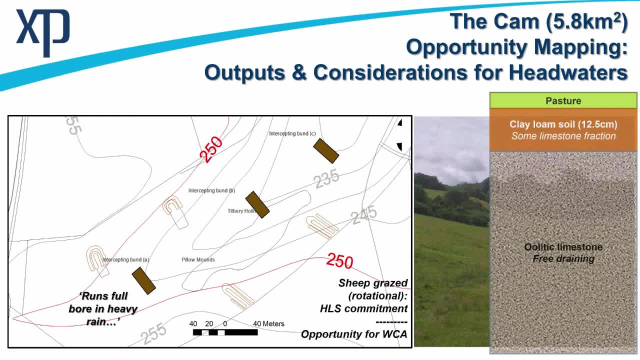 the area is underlain by a local substrate called Cotswold Brash, outlined, as I say, by this cross-section. Now, the designing of these schemes for modelling: it was important that bunds were able to allow for infiltration to this oolitic limestone. 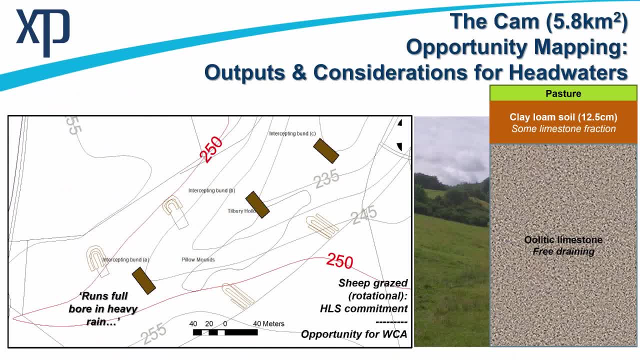 slowing the fast overland flows of the clay loam. Of course, in later modelling it would be important to consider the antecedent conditions in winter events and the existing height of the water table, to ensure we're not trying to infiltrate to an area already saturated. 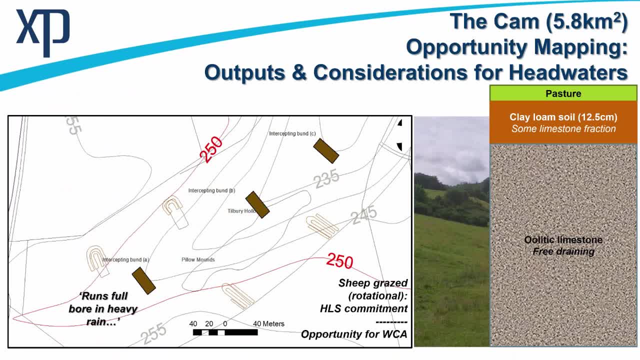 encouraging further flows. On another practical note, if you can squint a little bit, intersecting bunds B and C would allow for vehicle and sheep access in spate conditions, which was a very attractive proposition for the landowner in terms of evacuation routes. 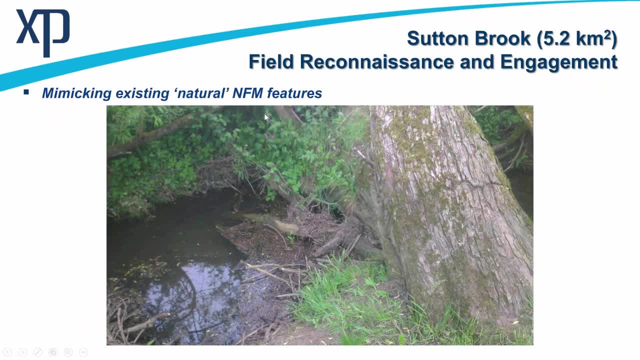 that Peter will discuss later Again. on a more practical basis, it's important to recognise these sorts of working with natural processes. features are aptly named so because they do mimic what is already happening in our catchments. This particular brook has a few existing 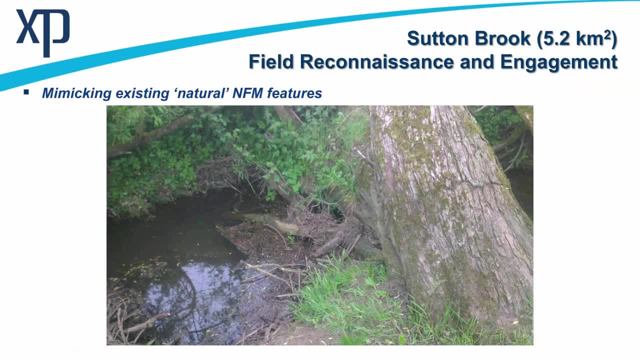 large wooded debris dams formed naturally but not removed by the farmer. This can be included in the base modelling that would impede and alter flow. However, on the ground, ensure that you examine the features in terms of how does it currently respond to heavy rainfall. 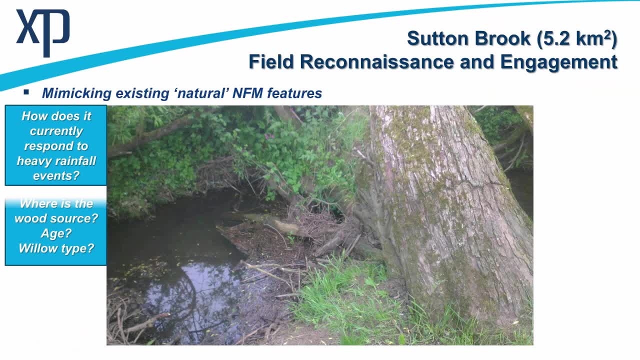 Is there considerable change in afflux levels? Is there a local wood source that's of a suitable age, For example this willow? can it be pleached to the bank to retain structural integrity? If you're with the farmer, ask if it impacts the business. 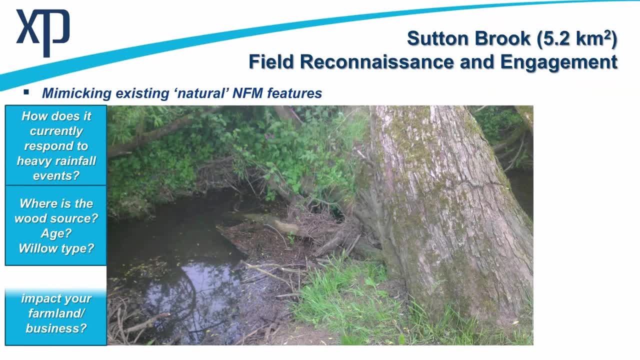 in terms of encouraging earlier avulsion onto a particularly productive crop. This is an important issue and looks well established, but nonetheless an important question. It's also important to consider what maintenance would be required, if any. Now, hydrologically, could this function? 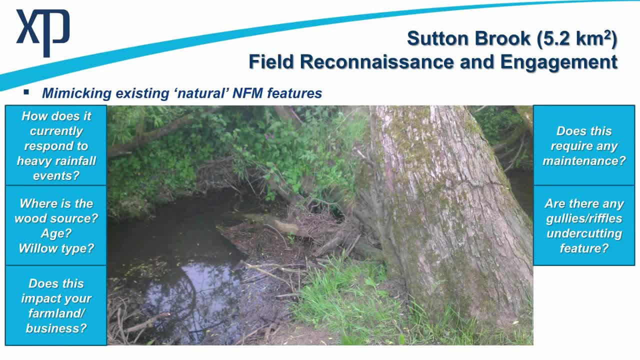 be altered with changes to the structure. Are there any gullies, riffles emerging where you want them to and not undercutting or eroding the bank? And, as I said previously, if you're with the farmer, ask if this sort of scheme. 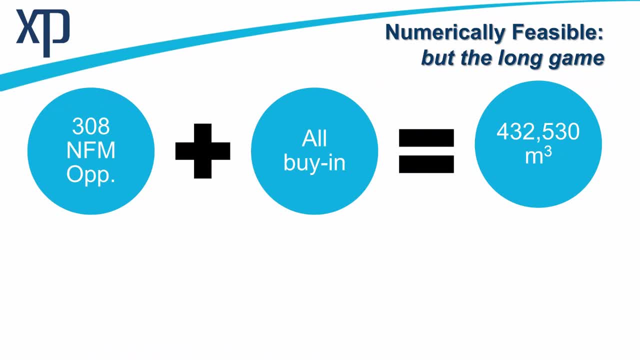 could be mimicked elsewhere. Now back to the MISO scale. 308 NFM opportunities have hypothetically the ability to attenuate 432,530 metres queued at maximum capacity when acting in peak events. Now this is using a ponding assessment. 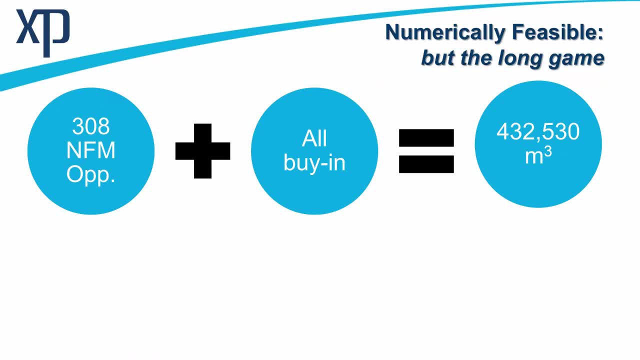 of conventional attenuation features and calculations of storage based on increased roughness and slope in terms of ruffling features such as forested water and retention areas, As well as ensuring all land owners and farmers consent to the works and designs. This is, of course, a completely 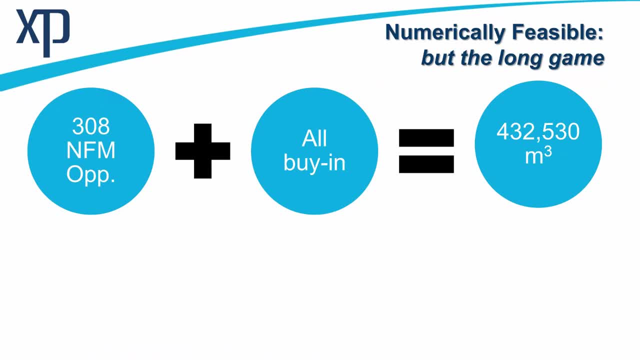 insightful figure, without considering model timing of peaks across isochrones of catchment and the impact of the storm flow in the hydrograph from different events. Because what we don't want to start doing is blocking all flow and creating a dam burst effect in which water 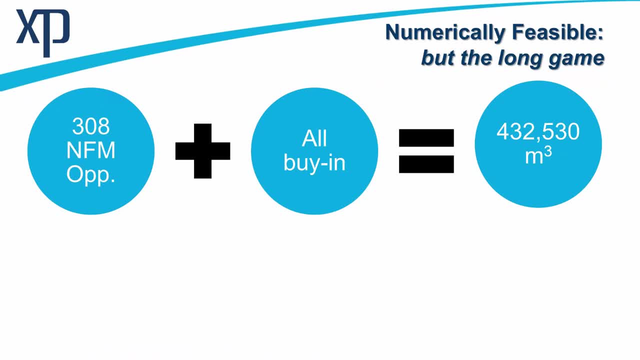 is synchronised in the hydrograph. We want to encourage slower through flow and continued base overland flow. Furthermore, this volume calculated is not water removed from the hydrograph, but the volume that would propagate through the system at a slower rate and lag time, attenuating the rising limb. 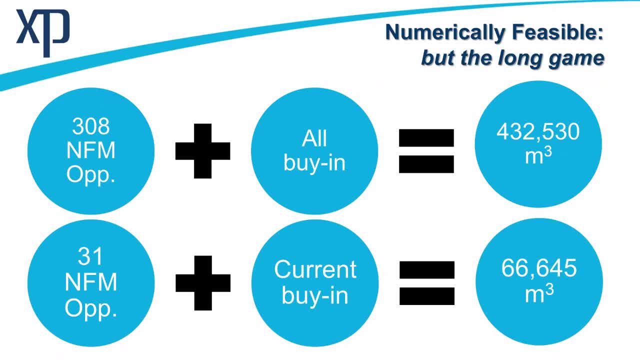 and a broader crested recession limb. Now what the second equation indicates is that, based on the currently consented and finalised landowner schemes that are seen to go ahead, these 31 features can attenuate cumulatively 66,645 m3. 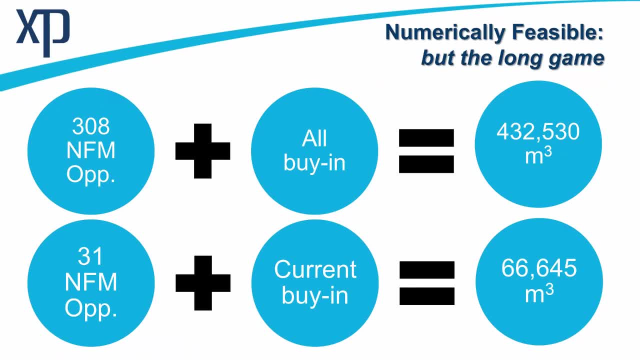 cumulatively 66,645 m3 each individually coming under the Reservoirs Act but obviously collectively having that attenuation capacity. This is 15.4% of the total design volume potential, indicating that this is a long game and requires supportive communities. 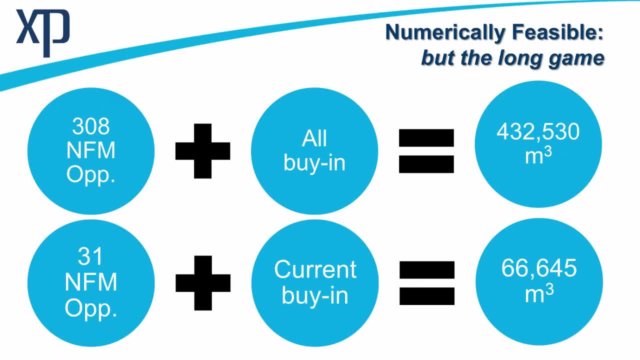 and farmers to drive this approach, when consultants and agencies and other contacts have gone. These calculations require validating through more detailed modelling of peakstorm hydrographs from contributing catchments and the overall required volumes to attenuate. that can raise a particular standard of protection. Now what I'd like to do now. 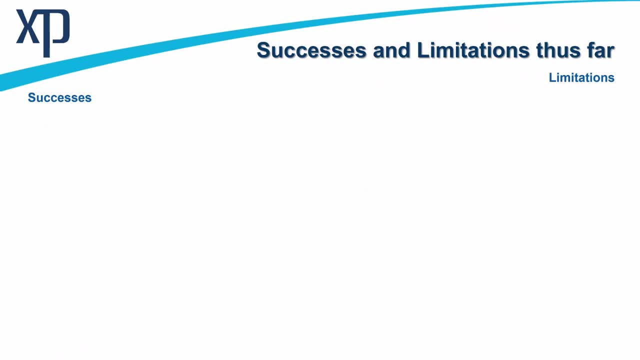 is. take you through some successes and limitations of the research thus far and how it can be implemented. Now. seven estates and landowners have approved NFM works and are looking to implement as soon as possible. One landowner has implemented six measures which I will show later. 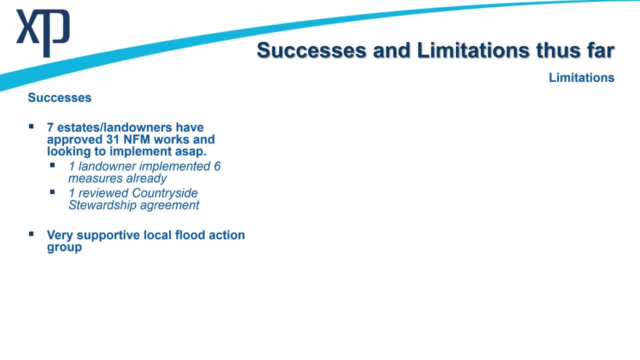 and there has been one reviewed countryside stewardship agreement. As mentioned previously, there is a very supportive local flood action group that helps mobilise the community around, taking ownership and also increasing their understanding of the flooding problems And, as I said previously, the majority of the catchments farming community. 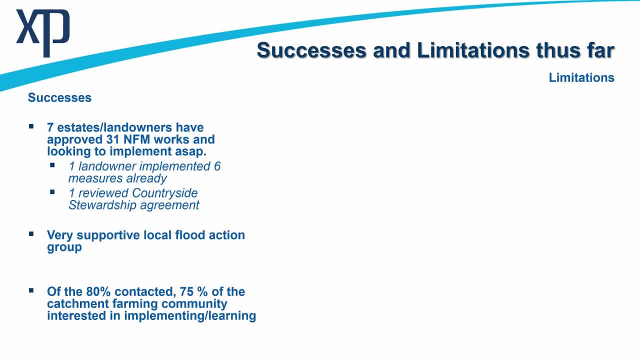 have been contacted, of which 75% are very supportive. I would also say the remaining 25% of those contacted are not unsupportive but need more convincing of the merits of integrated NFM across the catchment through more effective communication of modelled results. 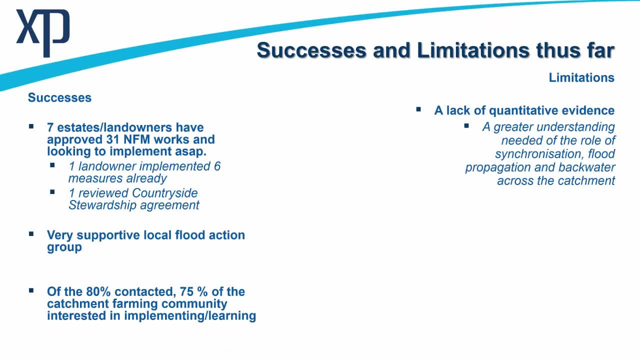 as well as further financial incentives. Now, in terms of limitations, as I'm sure you're aware of this research to date there is a lack of quantitative evidence around NFM at such a scale. There is a greater understanding of the role of synchronisation. 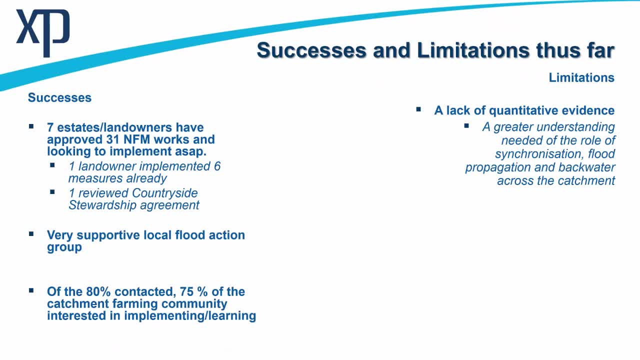 flood propagation and backwater across the catchment of the measures proposed because, as you noticed, there were properties also located upstream, Even though these features have been located with buffers of settlements. a greater understanding of especially these in-channel mechanisms is needed around the enhanced risk. 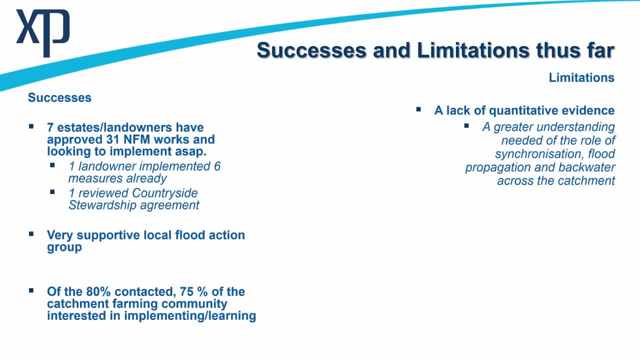 that could be proposed upstream. That's why initial pilot schemes that have been implemented have been carefully chosen as part of this approach NFM scheme. Now there seems to be issues with frameworks that make it difficult for local approaches to get off the ground. 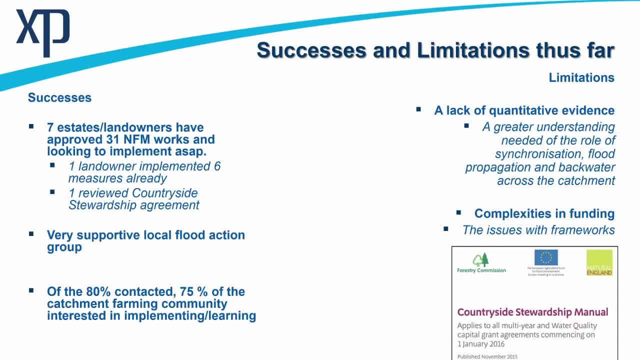 Principally countryside. stewardship has been very complex for farmers, and also the competitive nature makes it a slight gamble for them because they're having to invest time in an application that they might not receive any funding for, as well as flood defence grants and age. 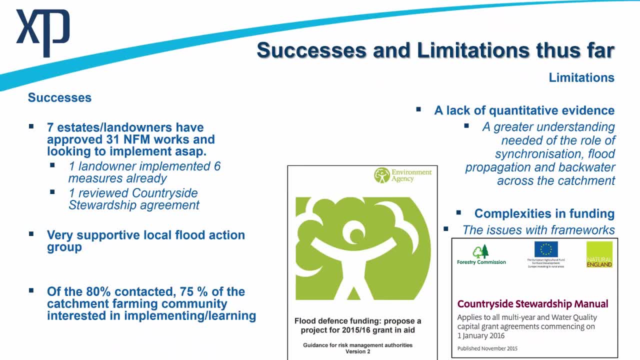 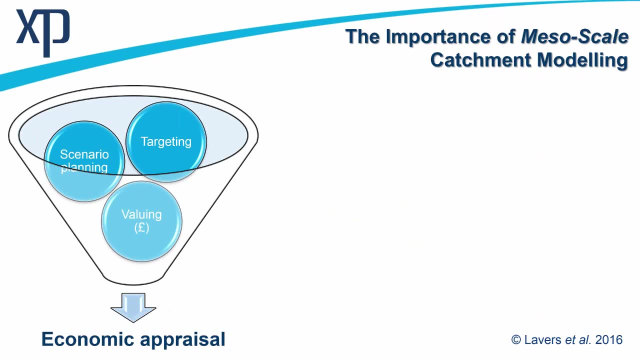 which fairly requires a decisive present value cost compared to present value benefits considered. NFM is iterative and highly dependent on buy-in, and obviously on a very large scale, and this can prove particularly challenging. Now I'll just quickly take you through the importance of mesoscale catchment modelling. 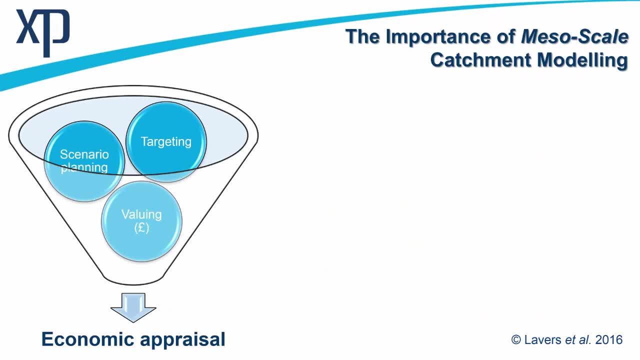 using the XBee Swim software. Now, understanding catchment systems is influenced by two fundamental characteristics. Firstly, identifying the storm flow as represented in the hydrograph. This is obviously the total volume of water present in the system that would otherwise not exist if the event had not happened. 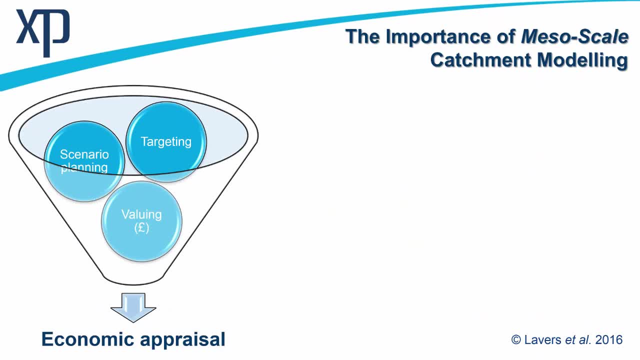 Secondly, identifying enough generation treated non-linearly, with time varying across the hydrograph. Now, the relationship between rainfall input and that lost or gained in the system is also key. so looking at evaporation losses, etc. Now these fundamentals of the XBee Swim model. 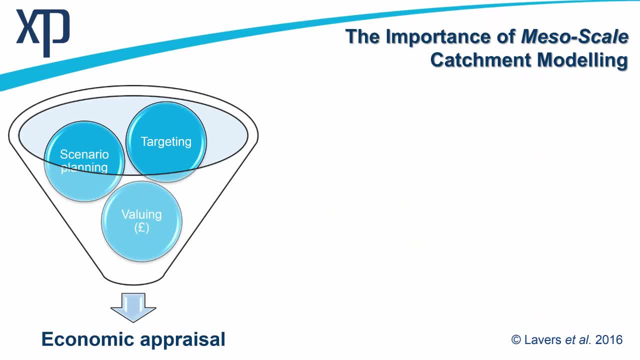 aim to inform three approaches that then give this economic appraisal that I'm going for. Firstly, it's important to target the most contributing sub-catchments, identifying the timing of peaks when delineated. Now, this allows for the schemes designed and mapped. 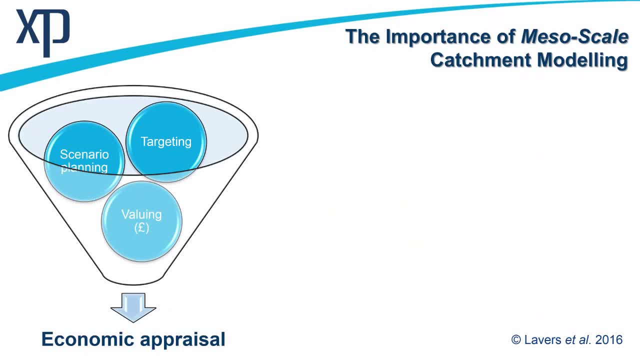 to be better understood in terms of desynchronising capabilities, as well as understanding the 2D influences that impact runoff generation, as similarly identified in the overflow model used by Durham University. Now XBee Swim actually allows for a combination of both these considerations. 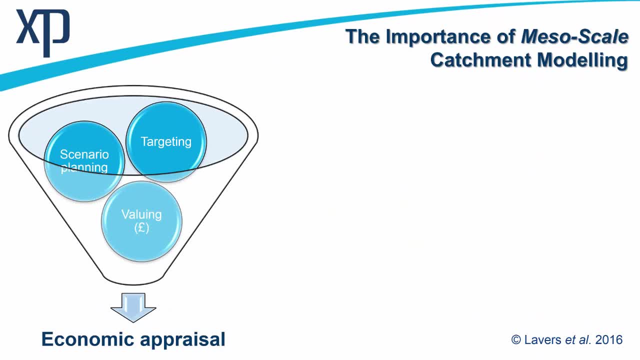 Then it's important to inform scenario planning, considering the ability of NFM features to attenuate downstream flood flows, understanding the base scenario and the resultant reduction in volumes downstream to different rainfall events. Now I've considered your bankful QMED scenarios: 5,, 10,, 20,, 75,, 100,. 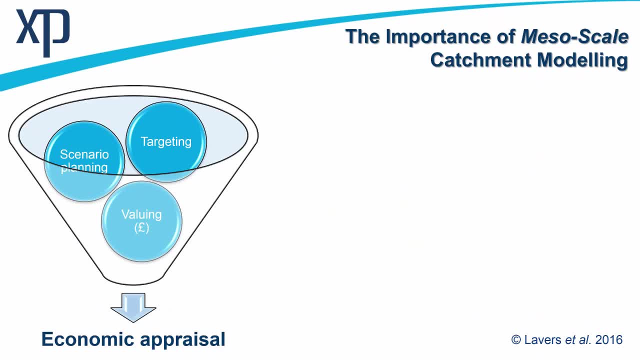 and, where available, the climate change allowances for 100 plus climate change. This can be input from FEH storm data with XBee Swim's built-in function with a recognition of a degree of uncertainty. Then it's important to value the scheme in terms of the reduction, if any. 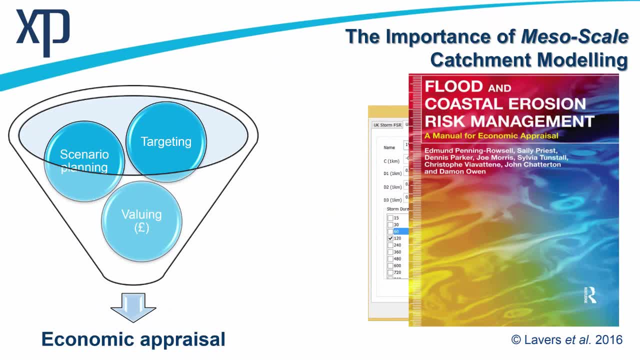 in average annual damages to properties and businesses. and the ability of the scheme to transition those exposed properties from significant risk to moderate, from significant risk to moderate, relating baseline risk scenario to NFM scenarios. Thus, what value is there in implementing an NFM scheme on such a scale? 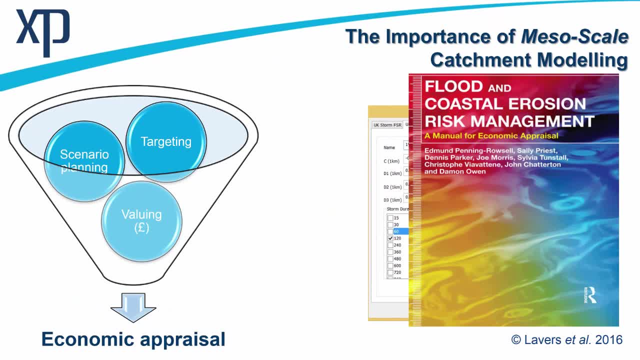 Now, based on the support from the network of landowners and farmers, XBee Swim's GIS-friendly outputs allows for a process of informal calibration. This can also indicate duration and time of inundation, which is critical for farm practices in that duration of flooding. 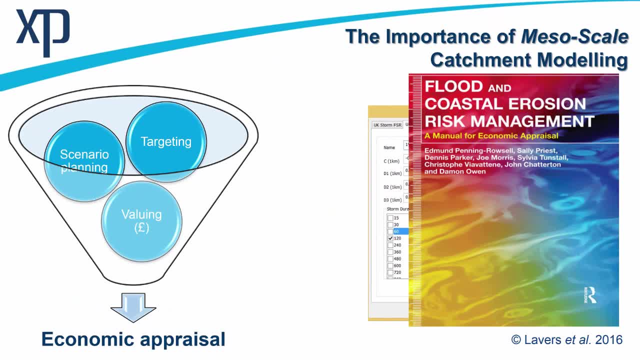 may help assess crop damage due to low tolerance for extended periods of flooding. therefore, using local knowledge to comment on model extents and depths and, if it matches their experiences and, ideally, images of the particular events, This exercise will also allow the model to provide present value. 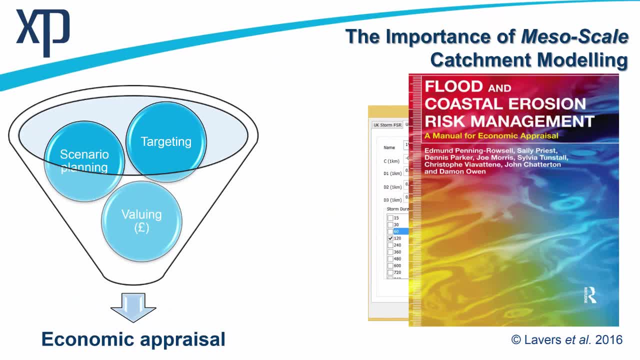 benefits of the scheme in accordance with the multi-coloured handbook that you can see associated with present value, costs and other studies, as well as the cost to the landowner with crop or corners of land being inundated. In most emerging studies, the NFM features are modelled. 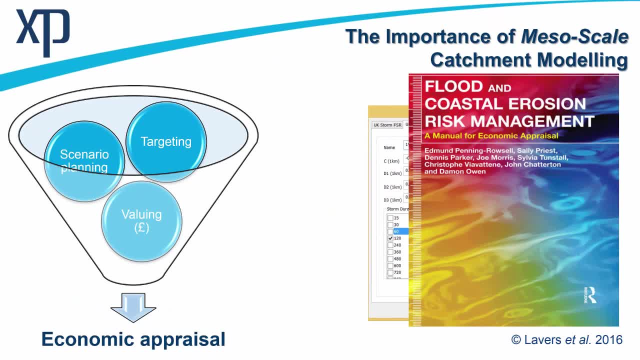 using different approaches and softwares depending on the function of each feature. Commonly, these are split into the corresponding domain. Those features designed to intercept 2D surface flow are modelled in broad catchment assessment techniques. Those features that aim to track the flow of water: 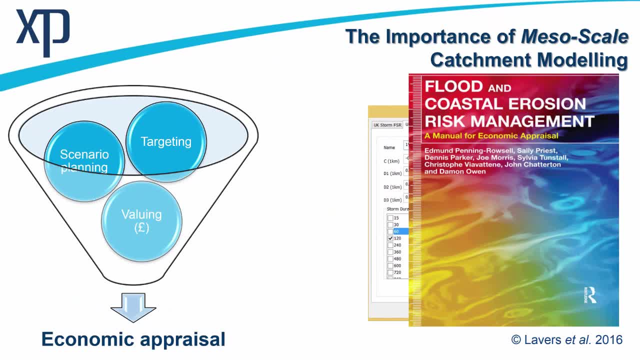 in the 1D environment are assessed using commonly ICIS2 flow models By the XP-SWM software linking two domains dynamically. this allows water to go between both environments and specifically give a greater representation of the 2D environment and the heterogeneous influences that can be altered. 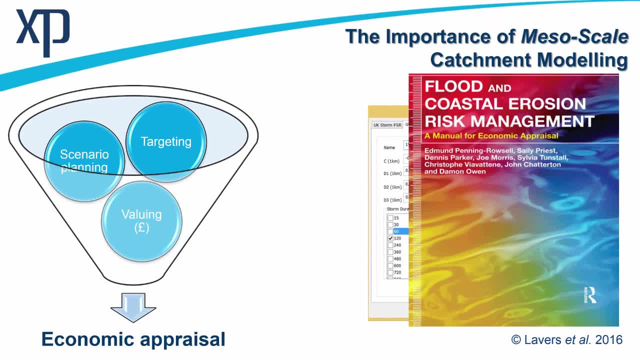 based on the map surveys, including things like existing hetero locations, As I say, 1D for this storage modelling and 2D for your routing and flood inundation modelling. These outputs are likely to alter the designs of the measures that I've previously discussed. 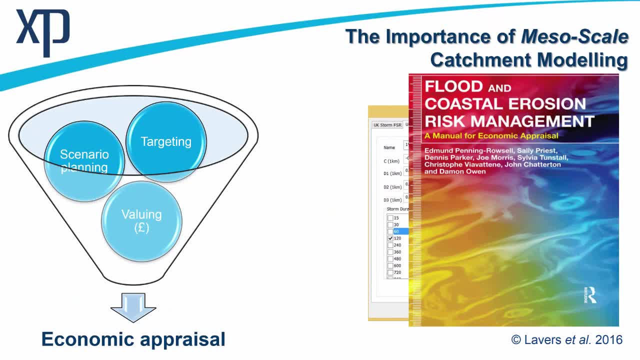 to ensure we're not augmenting the hydrograph in a way that prevents coinciding of peaks and maximises the measure's abilities across the catchment to desynchronise these flood flows. Now I'm quickly going to touch upon wider remunerations across ecosystem services. 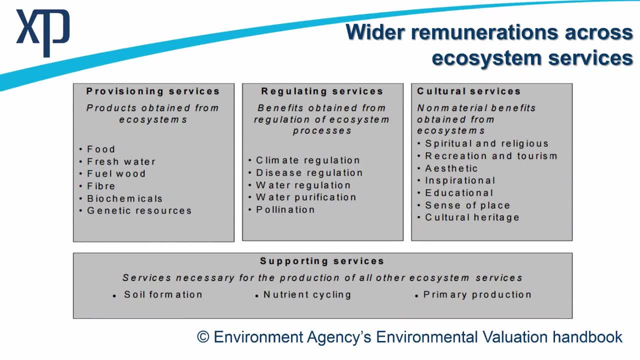 While this isn't explicitly part of the PhD, it's important to consider, especially from those backgrounds that aren't associated with modelling. Now, as commonly addressed in academic spheres, NFM is recognised to provide wider benefits across these ecosystem services. Most of these, if you're looking at, 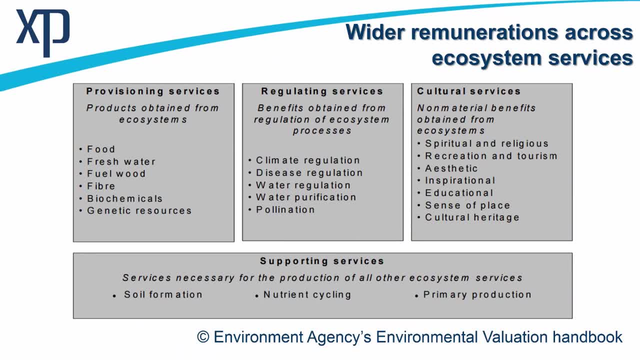 kilometres of improvement for water framework directed targets and habitat creation give an economic benefit to the scheme, associated with partnership funding calculators and stewardship payments. It's important to consult Natural England regarding these agri-environment schemes and or associated capital grants. These provide a further indication. 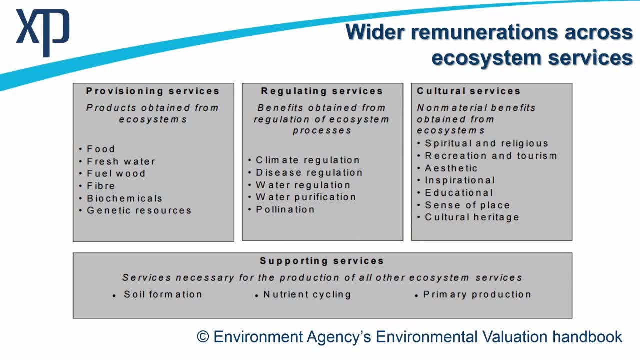 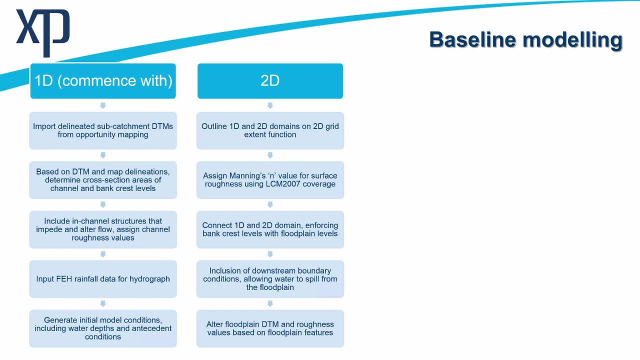 of the present value benefits of the scheme economically. Now this slide will take you through the construction of the baseline model prior the NFM scenario. that will not be discussed in this webinar due to some sensitivity issues, as well as the infancy. But firstly, it was important to commence. 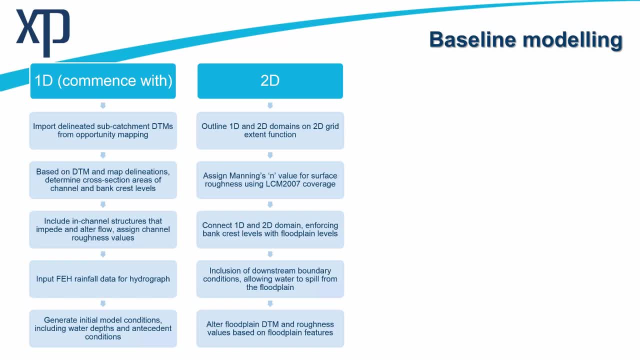 with the 1D model build and importing, delineating sub-catchments from this opportunity mapping phase and ensuring discretisation of the whole catchment with the associated strata order and the contributed catchment terming, cross-sections and bank crest levels. 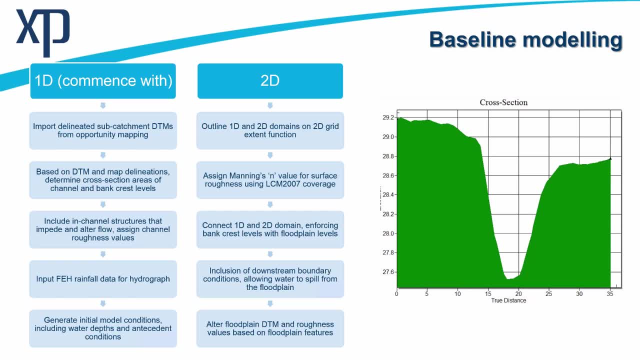 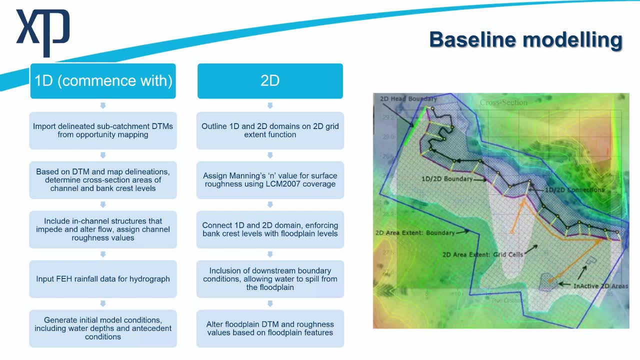 This includes in-channel structures that could impede flow and water flow, including weirs, existing debris dams, and assigning channel roughness values based on the type of water course, Then it's important to input this FEH rainfall data that's available to DSA. 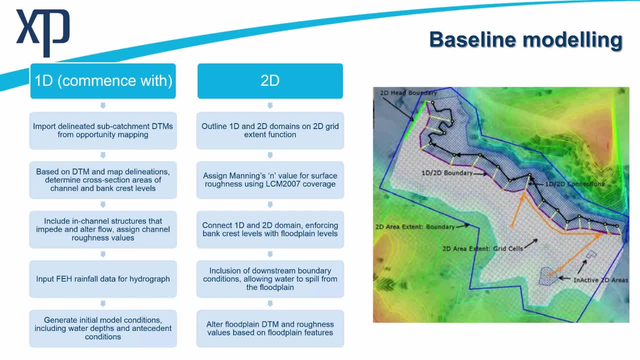 this data is a 1999 source- and then generate return interval storms. Of course, there is a real issue with associated validity of this sort of data That these are not directly calibrated to return periods therefore need to be sensitively analysed in terms of volume errors. 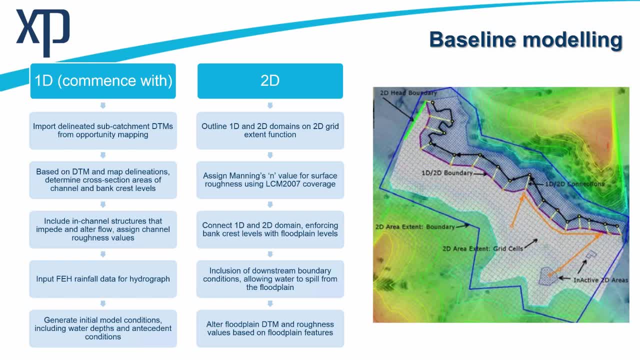 relating to the one-stage discharge monitoring station that I have at this catchment, Then it's important to generate initial model conditions, including water depth and outer sitting conditions, Then incorporating the 2D domain, outlining the 1D and 2D domains on a 2D grid extent function. 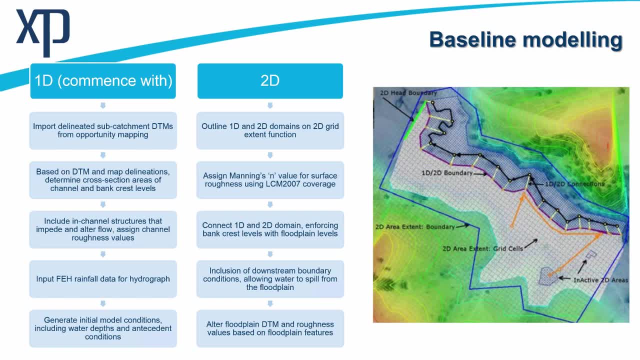 as you can see. then assigning Manning's n-value for surface initial roughness: 2007 coverage, as you can see here. then connecting 1D and 2D domains, enforcing bank crest levels with floodplain levels. Now, this is an interesting consideration when assessing features that force. 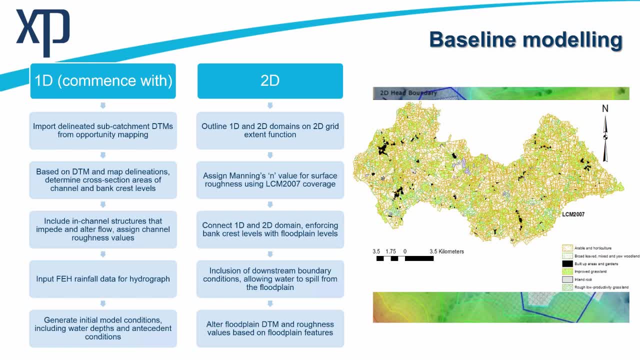 evulsion at earlier rates, increasing volumes and levels on the bank of the river network, such as enhanced debris dams- not just your conventional smaller ones- or points of enlarged online and offline ponding. Inclusion of downstream boundary conditions is then followed by floodplain DTM and roughness values. 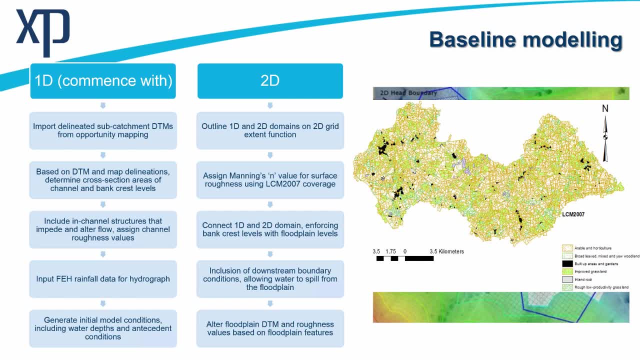 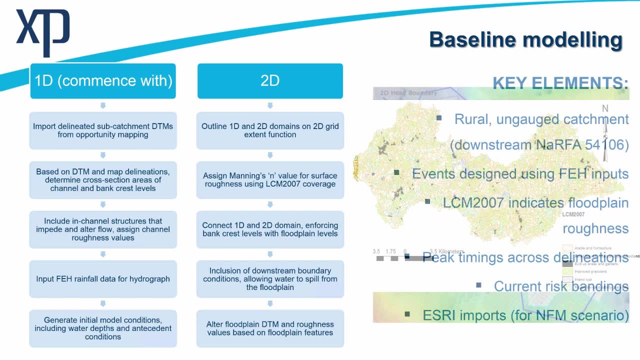 based on pre-existing features such as your outbuildings and head roads. Now, as part of this modelling, I think it's important to recognise the catchment is mostly engaged with no validating monitoring equipment, with the exception of the downstream node gauge that is past the confluence of the headwaters. 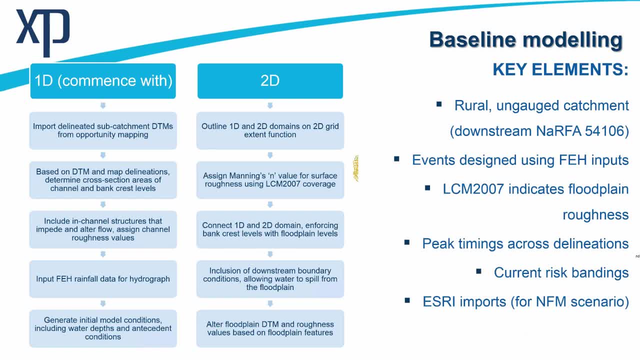 Therefore, a great deal of uncertainty must be recognised and calculated with the modelling, including storm events themselves, from this FEH data. A lot of past research on larger catchments have highlighted the importance of synchronising flood flows. therefore, timings must be carefully considered on attenuating that sort of hypothetical. 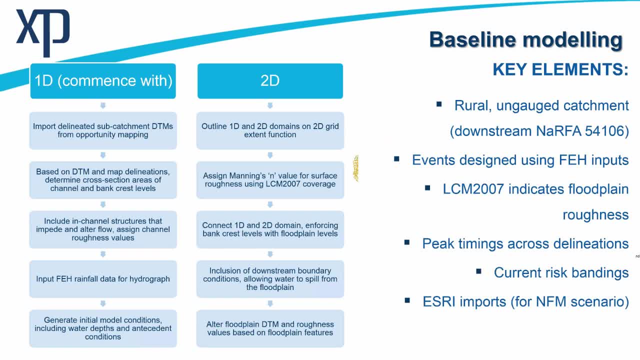 432-530m3 through the system. This utilises the unit hydrograph as a routing component of the catchment model in XPSWIM software, based on how long each sub-catchment will take to reach the outlet that ships engage and how the hydrograph is fundamentally augmented. 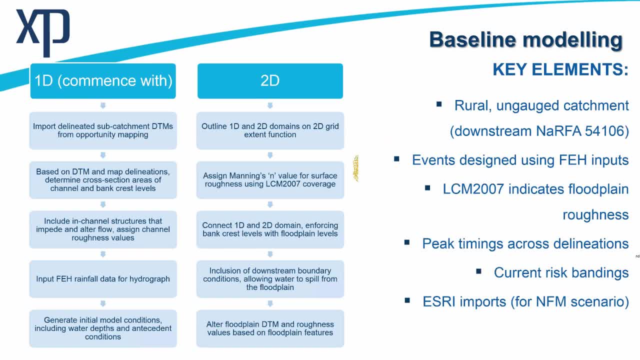 Also. ultimately, this research aims to indicate a transaction of risk bandings between companies and businesses. Therefore, understanding current level of risk is key in the initial assessment of this particular base modelling. Now I'll quickly go through a summary here before I pass you on to Peter. 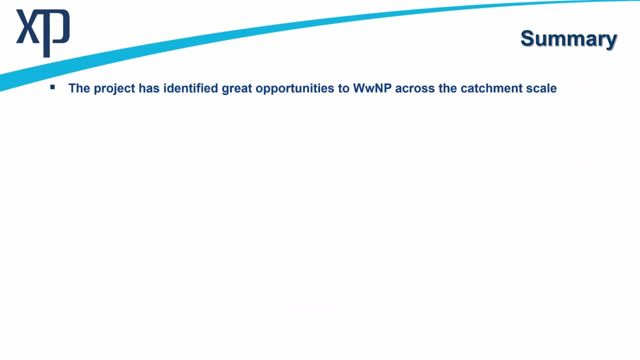 But the project has identified great opportunities to work with natural processes across the catchment scale. Partnership and interest in the evidence has been key to the success to date. There are practical and numerical issues and questions that need to be addressed with NFM because there is a lack of quantitative evidence. 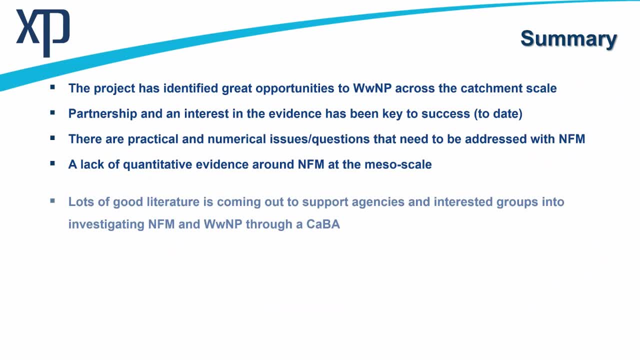 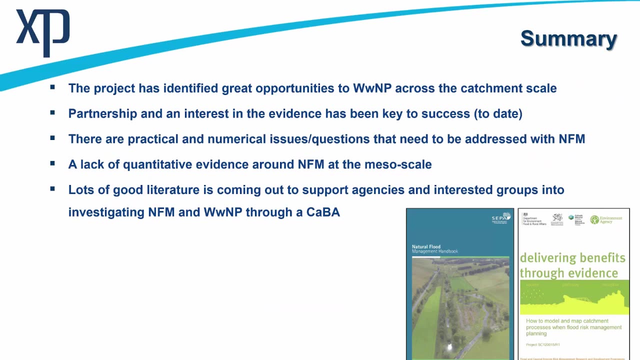 around natural flood management at this sort of scale. However, there is lots of good literature coming out to support agencies and interested groups into investigating NFM and working with natural processes through a catchment based approach. Examples included here. However, I would like to finish off. 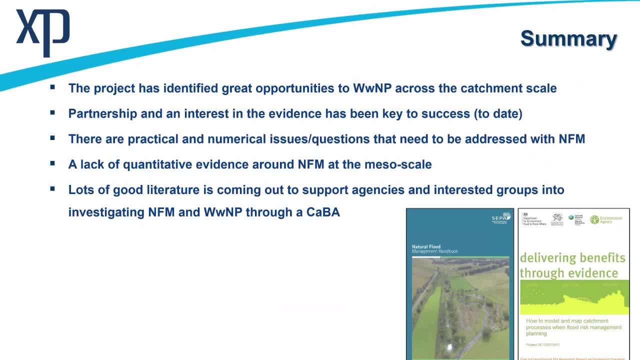 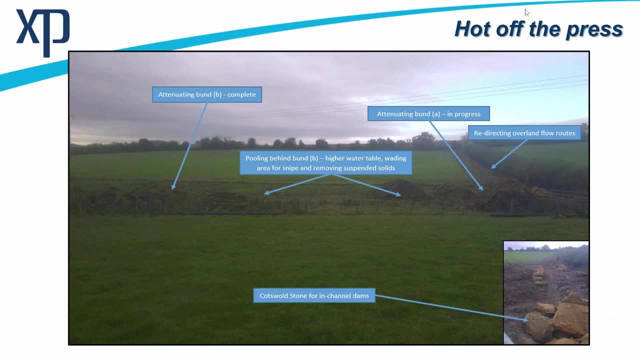 referring to the 27th recommendation in the pit review and that we need a suite of measures to manage flooding. By no means am I suggesting that there should be a plan that adapts the services of our catchments. Now the image shows measures that have just been implemented. 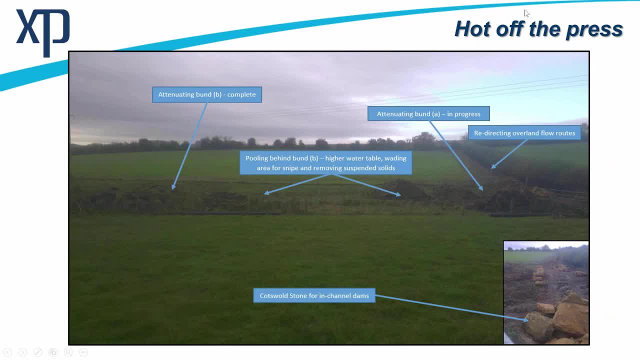 excitingly, in the Knee Brook You have two intersecting bunds that are designed to attenuate pluvial flow entering the brook in peak events, with flow going from right to left and the receiving watercourse being about 220 metres down. The scheme also includes stone debris. 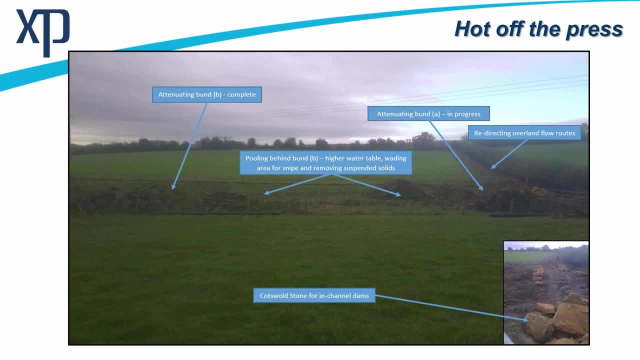 to act as in-channel dams to slow a particular pond outlet using local Cotswolds stone. This means that the source materials keeps costs down whilst trying to perform the same hydraulic function as would large wood debris dams. This scheme also includes the ditch management of neighbouring farmers. 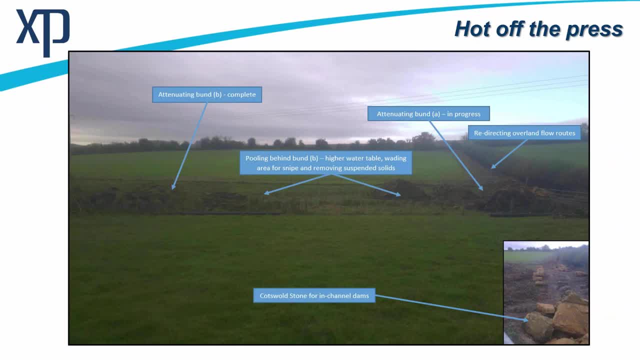 who have agreed to incorporate their ditches with the bund scheme, attenuating basically two farms for the price of one. This view indicates the cross section of the bund and it's been footed into the substrate at 1.5 metres high with a 9 inch orifice. 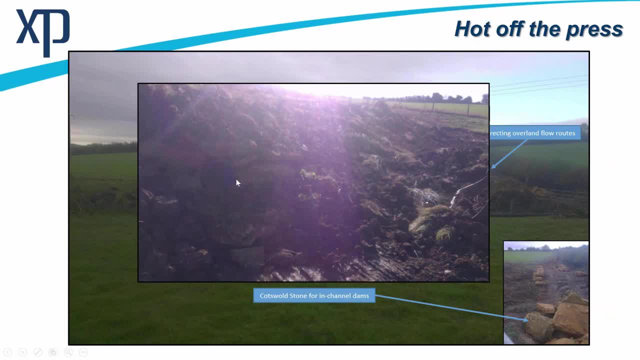 To counter the venturi effects, we have implemented a right angled inlet to slow through flow and encourage further attenuation in these peak events, while still allowing base flow to continue. As you can see from the bund, the topsoil was removed carefully by the farmer and then reseeded to ensure grass. 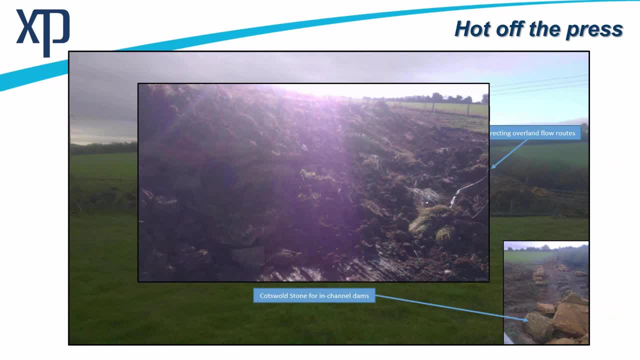 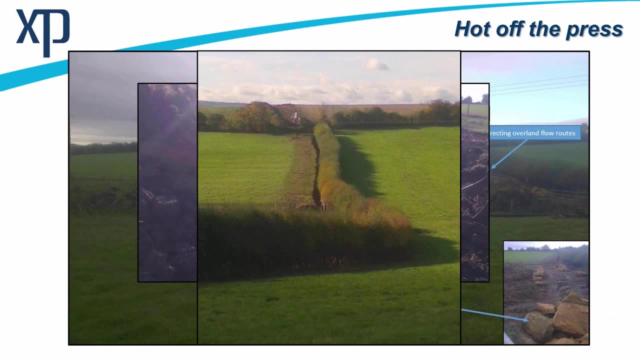 could seed and then hold the bund and prevent erosion. This image indicates the redirecting ditch behind the first attenuating bund. It's also worth noting the raised water table and bund mechanisms aim to increase saturation and habitat improvement for common skype and they are a targeted 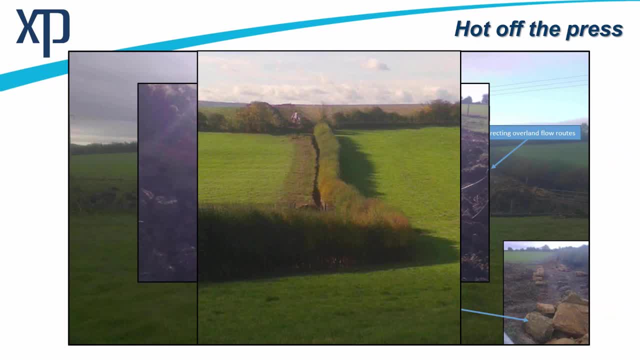 wading farmland bird for the Warwickshire Avon as a whole. These measures also drop out silts and binding pollutants, mainly pea, from the pluvial flow before it enters the watercourse along this steeped conduit of farmland. This farmer is by no means. 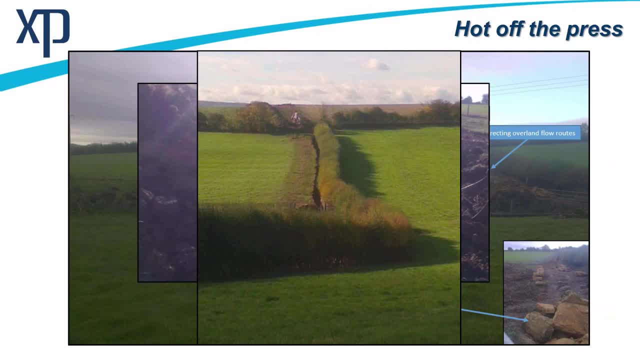 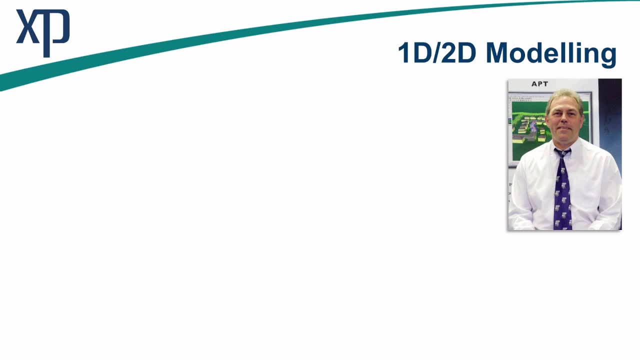 currently farming in a way that encourages diffuse pollution, but he recognised the opportunity to grow more flay. Now what I'll do is just pass you over to Peter to finish off the presentation. Thank you, Tom. that was really interesting and engaging and I hope that's. 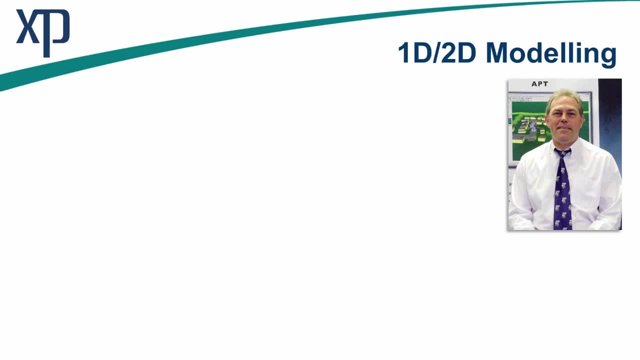 opened up some possibilities for the audience at large here to see what we're actually achieving already, and very much is infancy, but a great start and I very much look forward to keeping everyone up to date with Tom and progressing the case study over time. So, looking at the modelling aspects, 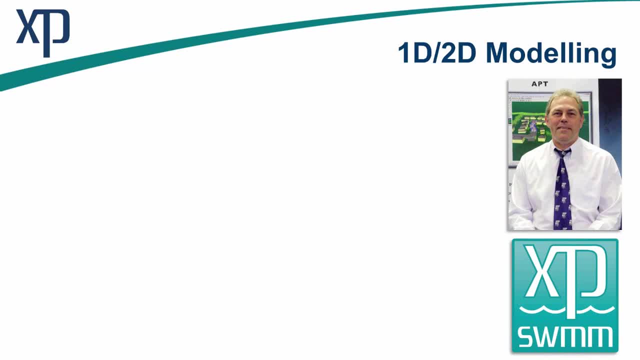 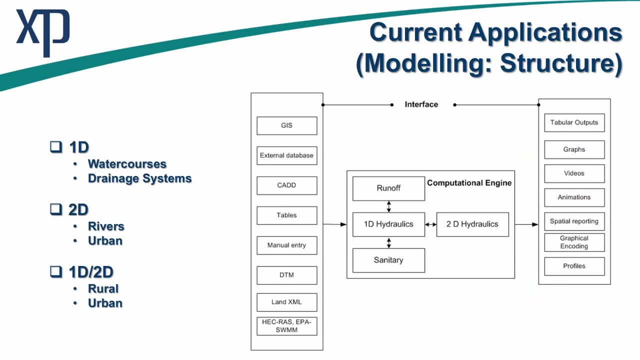 and what we're doing and where we're going through the use of the XP-SWMM programme, our modelling software, which is being used on this particular scheme. What we've been doing historically for the last 30-40 years with XP-SWMM is modelling a range of things. 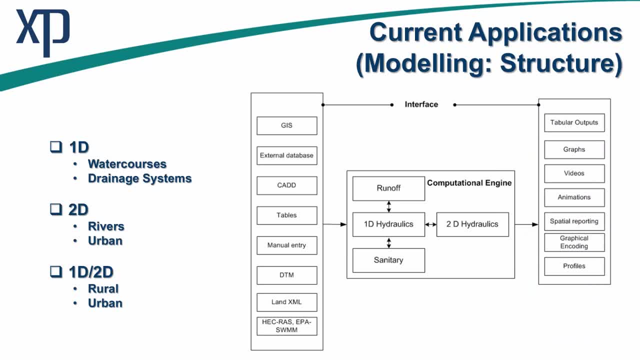 whether that be watercourse drainage systems in the urban environment, in the rural environment or mixed- and often we get asked the question: what should I do? What's the best method to go forward? Should I use 1D? Should I use 2D? 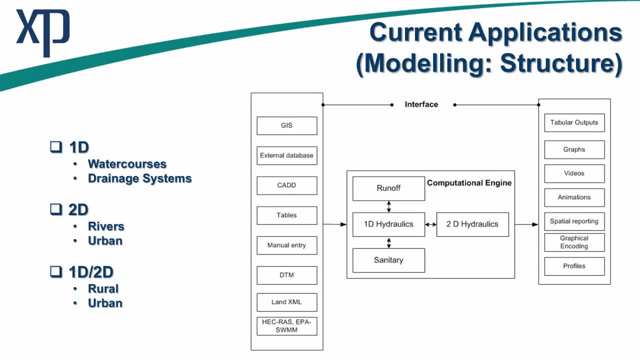 And what we're looking at on this catchment scale is the best of both to get the best of both worlds. basically, On the left hand side, here you can see all the various inputs that Tom's kind of mentioned: GIS inputs, bringing in terrain models to create surfaces, and topography. 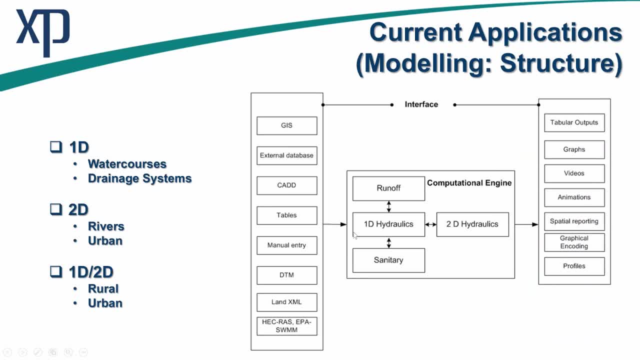 set up the base scenario. so we have a range of inputs coming into the programme and we run with computational engines. for the 1D, hydraulics, we're using, as I mentioned earlier, the EPA SWMM engine, and then, when you have surface flooding and we go to the 2D domain, 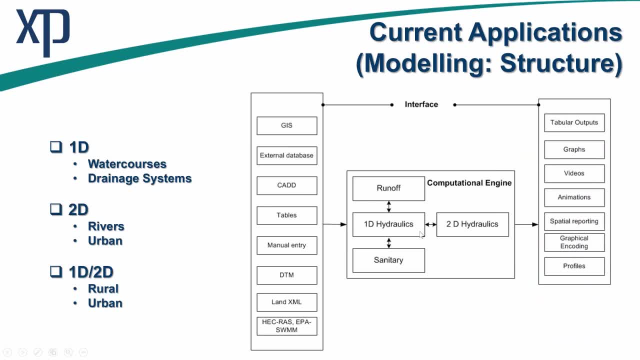 we're using the 2Flow engine, so it's a combination of both. and this is where the programme comes into its own, because it provides this user friendly interface to enable you to grab whatever information you have from sites. you can also incorporate any missing information, go out, survey, talk to the locals, etc. 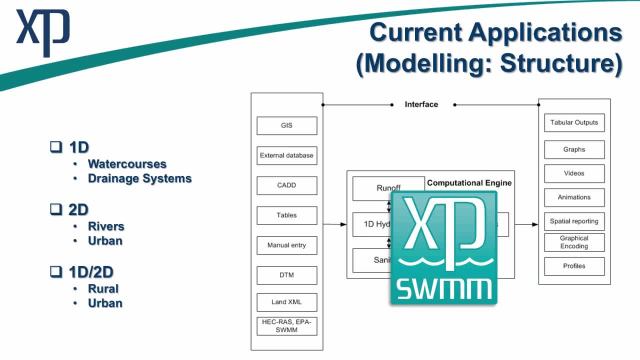 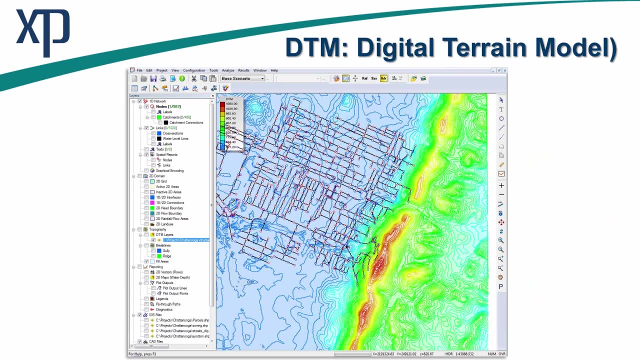 and enhance that model to get a good base scenario. and, very importantly, on the right hand side, we then need to express the results and look at the various options that we're considering and provide those outputs in a meaningful way that we can share with all the various stakeholders. 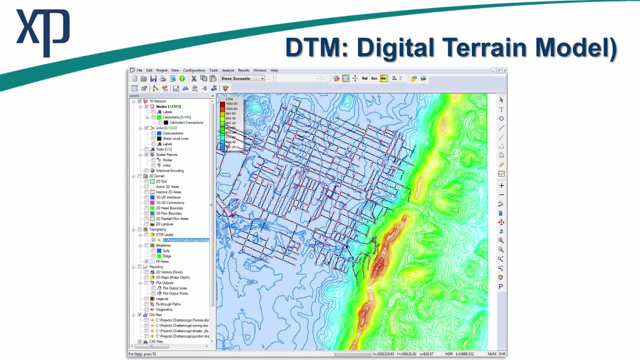 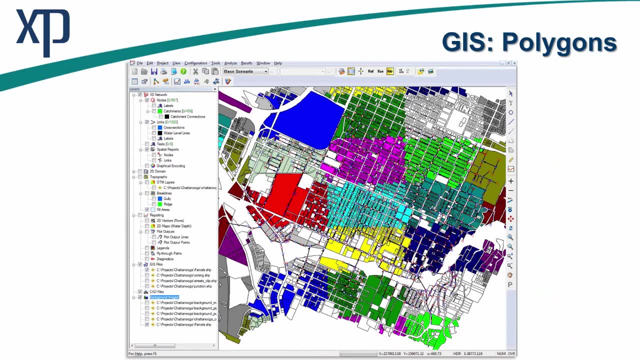 so, to start off with, we bring in a digital terrain model, and this could be the lidar data that Tom mentioned, that has been provided by the Environment Agency. upon that terrain model, we can then import the GIS data, so looking at various land usages, crop usages, etc. 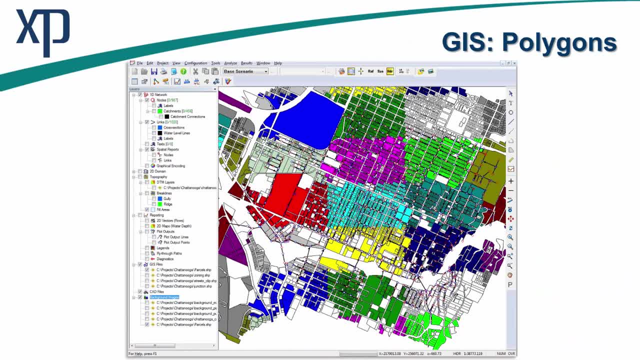 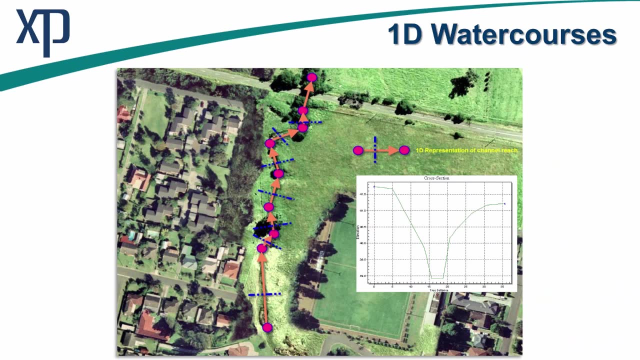 maybe highways provide the various roughnesses upon the surface by creating those from the GIS polygons that are imported. we then start looking at the more detailed aspects that would influence the model more greatly, such as the major water courses, and here we could well, if you have a headcrest model. 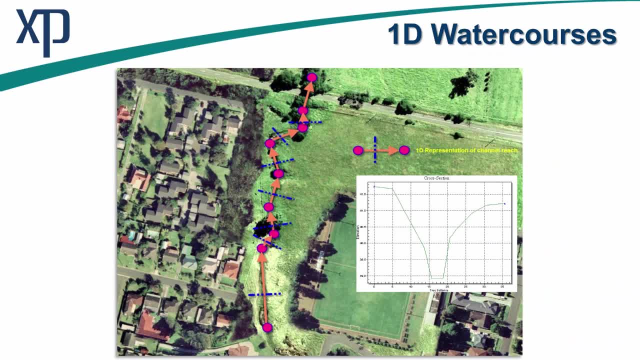 for example, we could import a headcrest model or an ISIS model. if you even had a drainage system, you could import the micro drainage system if you're looking at an impact of a development upon a water course, for example, in the absence of any information, worst case scenario. 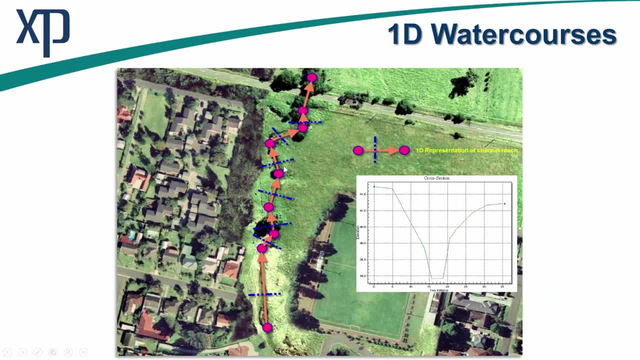 we could cut cross sections from the lidar data. this may not be the most accurate, but we could cut cross sections midway along the links. so we'd set the water course up as a range of links and intermediate nodes. so when the cross section of the water course changes, 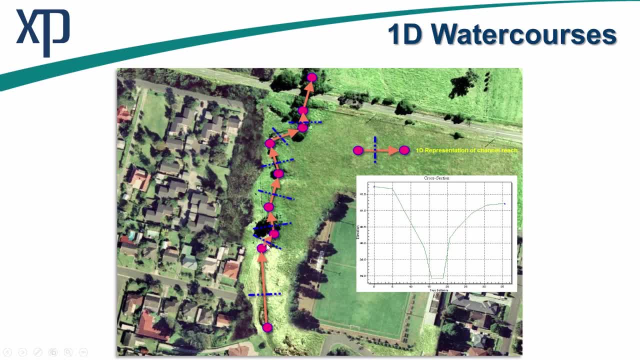 then cut a cross section at the midpoint along the link and then have a series of these shown on the right hand side here. so we have reasonable data. or if you go out and carry out a survey, we can import that survey data and provide a very accurate. 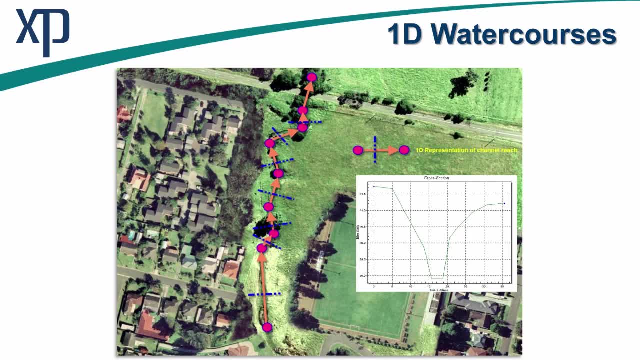 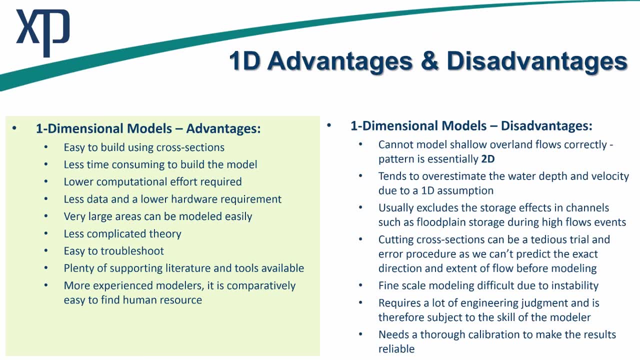 cross section as measured now if you were working just in 1D. there are a range of advantages but also a range of disadvantages of just working in 1D. historically, this has been probably the more common format that people have been used to working with. we've got a lot of good quality engineers. 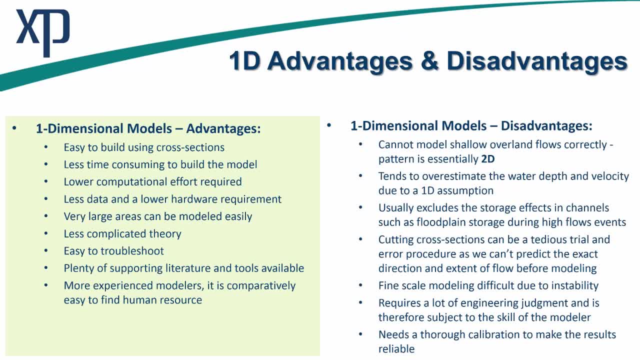 out there who can very quickly set up these models. there's not a lot of computational effort required, but you do require a lot of engineering judgement to set these things up properly. so there are advantages and disadvantages. I'm looking at the time so you can quite happily read through this. 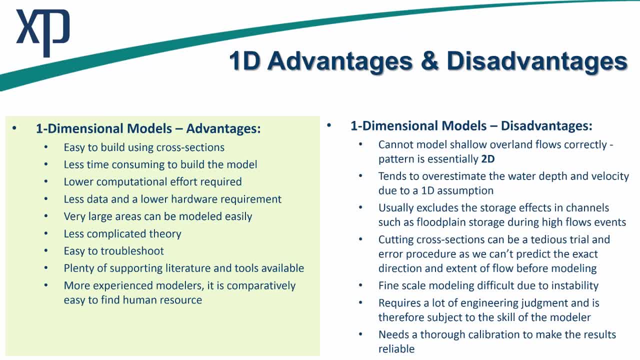 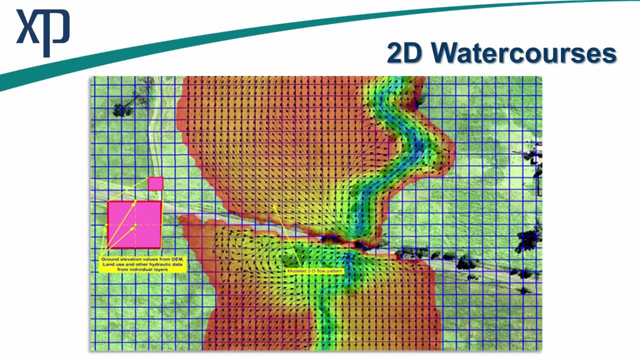 in the recording that I'm making of this particular presentation, or just email us and we can send you the presentation directly to you as well. you could work purely in 2D as the other option. the issue arises here on scale of a very large area, so we would set up some very large grid squares. 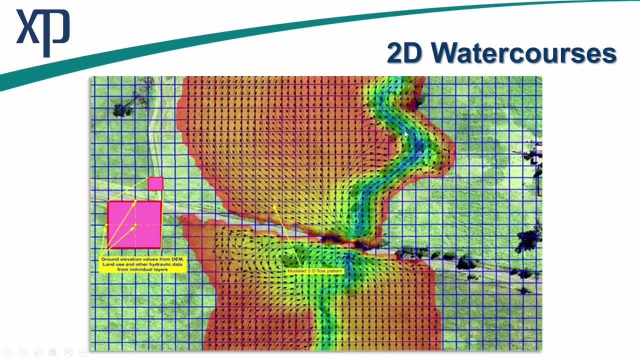 for the rural areas, but then when you get down to the watercourse information, you'd need to have very much smaller grid square sizes and on such a grand scale. to get this accurately established in, 2D could be a stretch, so the idea would be to use 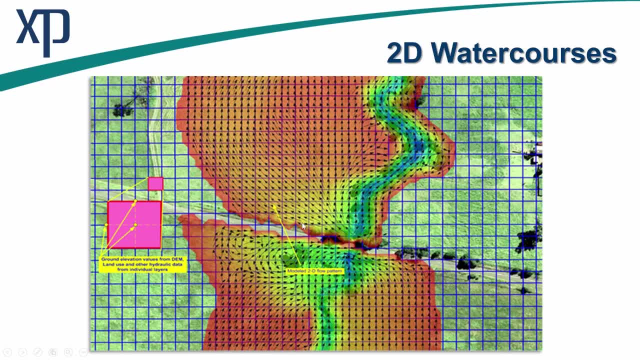 the 1D methodology for the watercourses and then apply the 2D when the watercourse is in flood, when the water is topping the bank, and this is the methodology that we're incorporating within the Shipston case study. again with 2D. there are some great advantages. 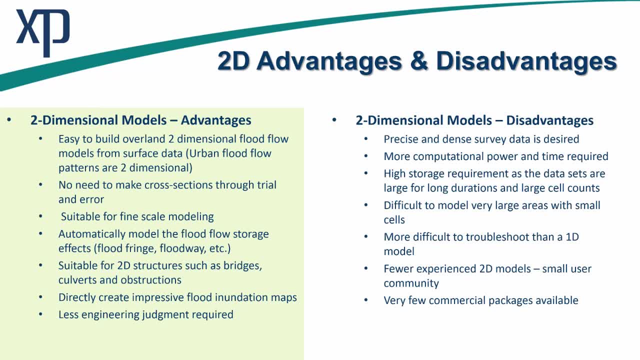 but also some disadvantages of purely working in this mode and we don't have so many people that have been using the 2D in this country. it's growing and it's growing quite quickly, but there are few and far between experienced 2D modellers. 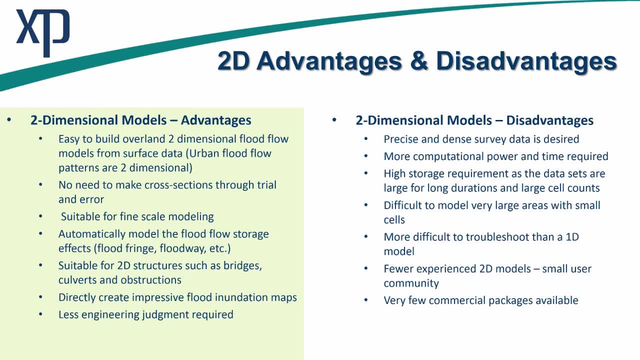 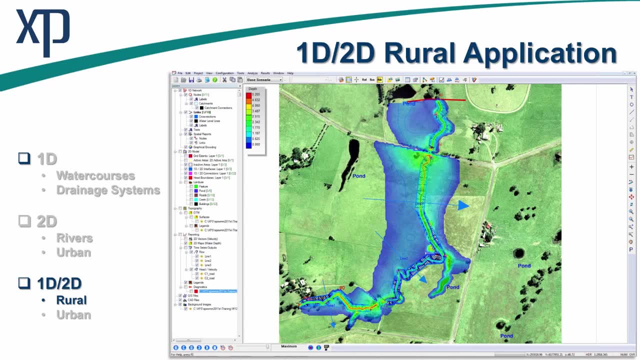 and there aren't that many packages that are commercially available as well to carry out this type of work. so we're going to test both worlds and set up the watercourses in 1D and then analyse the overland flooding in 2D, and this is specifically for a rural application. 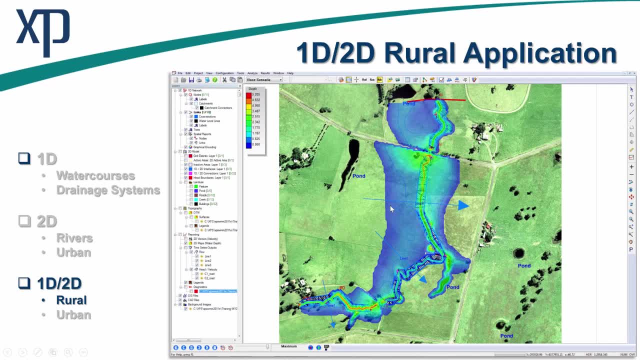 the amount of detail that we put in here is purely down to the site conditions. so there are no concerns. if we have a road crossing with a culvert, this can be modelled. if we have a watercourse with a bridge, this can be modelled. we can have ponding areas. 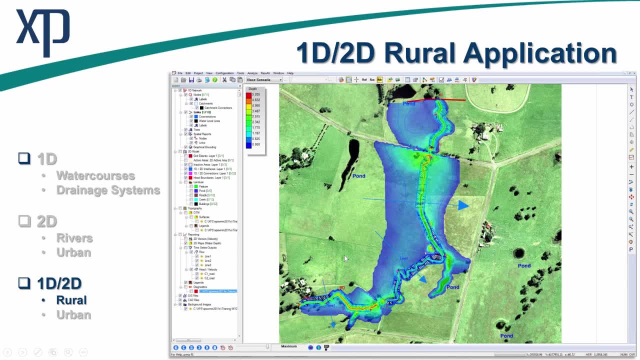 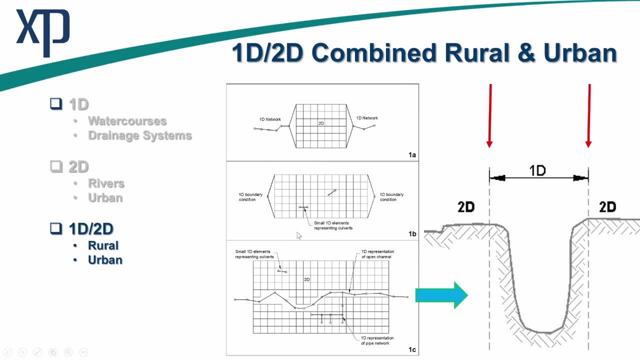 within the DTM, woody debris dams, etc. all within the software itself to create this, initially the base scenario. when we're looking at the 1D- 2D combination, this is really illustrating what we need to set up in the model we set up the watercourse in 1D. 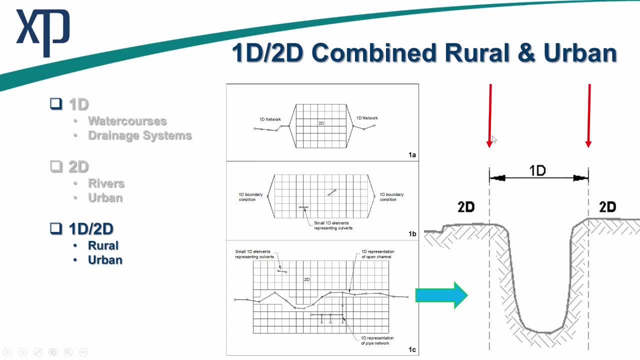 we would establish, looking downstream, the left hand bank and the right hand bank. so to convey the flow and analyse the flow, the most accurate way really is within the 1D hydraulic section. what happens when the river bank is in flood? where is the water going to run? 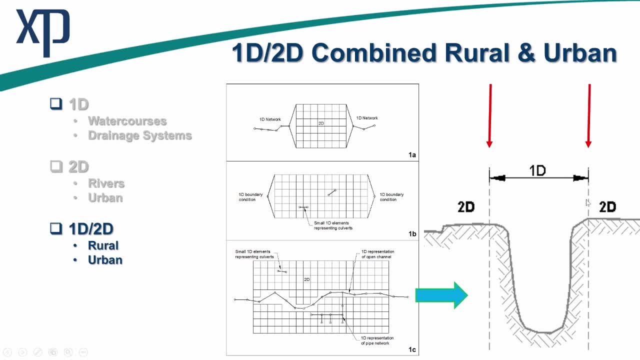 across the DTM and this is where we need to establish the connection between one and the other in the model and then analyse, without double accounting, for the flows within the model itself and, as I mentioned before, with this watercourse we could set up a base scenario. 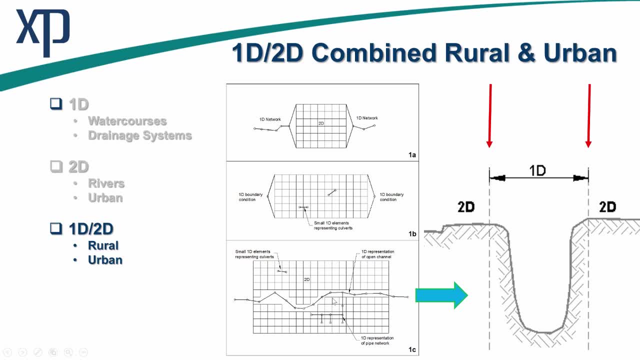 with a watercourse, if someone was working with micro drainage and designing a new development that connected into a watercourse, along with the subcatchment areas that are creating the flow within the new development, to look at water levels in the river itself. so that's another option. 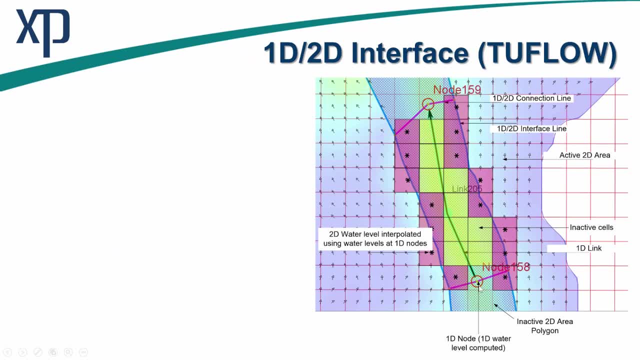 for working with the programme. so, looking on plan, what we would do is set up connections between the 1D and the 2D and have an interface line along the right hand bank and along the left hand bank. typically we would set up our grid squares. 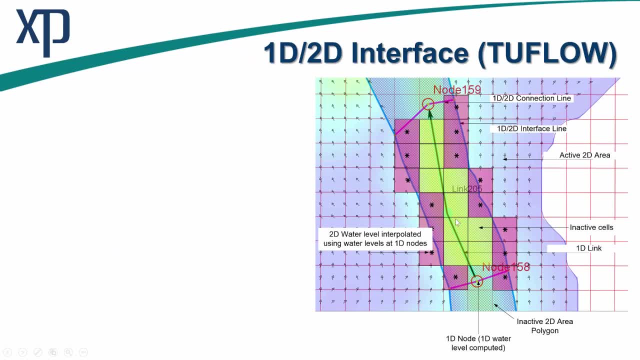 as I say, more dense in areas of known flooding issues and larger grid squares for the large expanses of rural area. and that's important because if we were working just in 2D, you could use a very, very large grid square and basically miss the impact of the cross sectional. 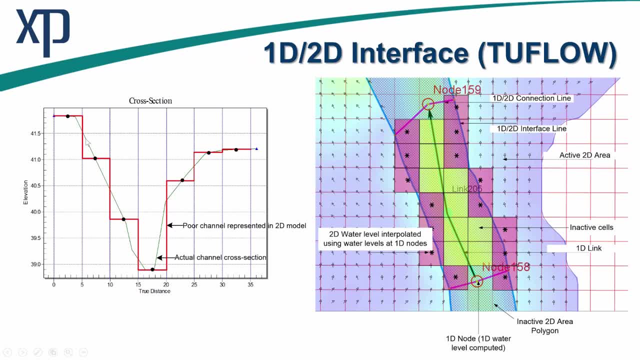 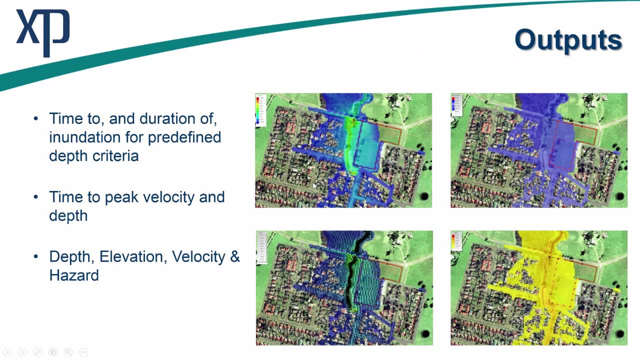 area of the watercourse and that watercourse may simply be ditches along hedgerows and things like that, which could have quite major effects on the runoff characteristics of the catchment. and then, moving on, once we've run the analyses for those various return periods and including 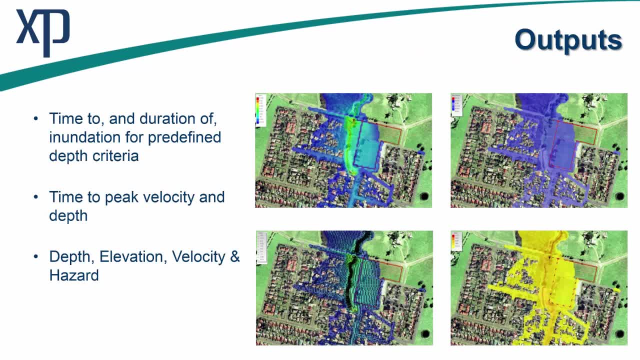 climate change. as Tom mentioned, we can then output information in a variety of formats, and this is really important in terms of sharing that information with the stakeholders. we're looking at times and durations of inundation. this would be specifically important for those crops. how long are the crops under water for? 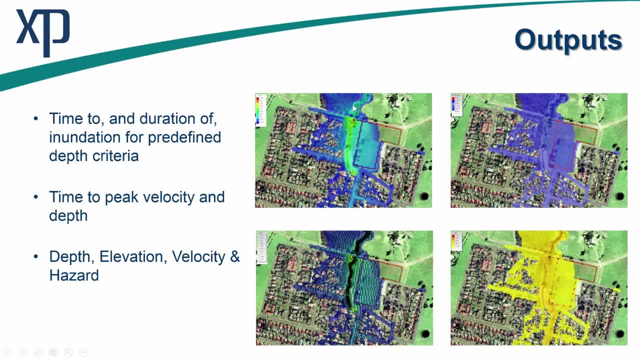 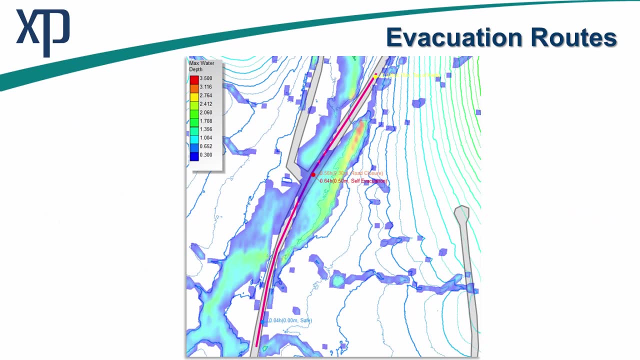 what's the velocity of the water? what's the depth of the water? how long would it be under water? for how long until that water reaches its peak velocity, peak depth, and a variety of different outputs that we can extract directly from the programme, having run the analyses. 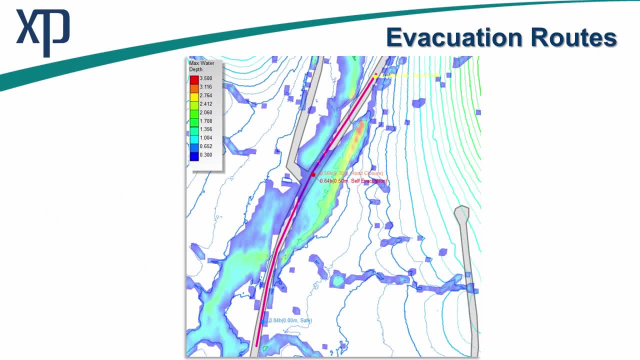 so we can set up a base scenario. we can then set up a range of different mitigation measures. we can look at identifying a range of ideas, implementing those ideas into the model and then running the analyses simultaneously and then comparing the results. this is just showing you another option to extract information. 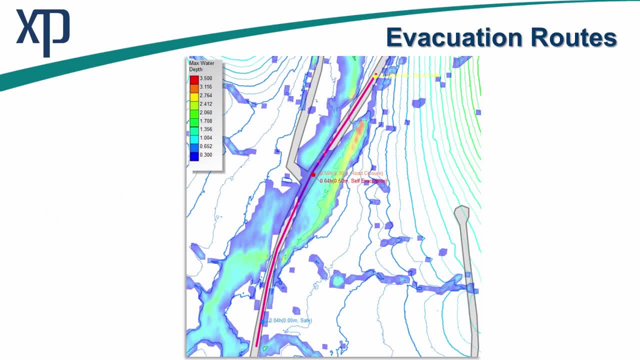 based on evacuation routes. so Tom mentioned the, the buns idea, and when the buns are holding back the flow, with the nine inch orifice or the nine inch pipe running through, those buns themselves become evacuation routes for the sheep to cross from one field across to the higher land. maybe. 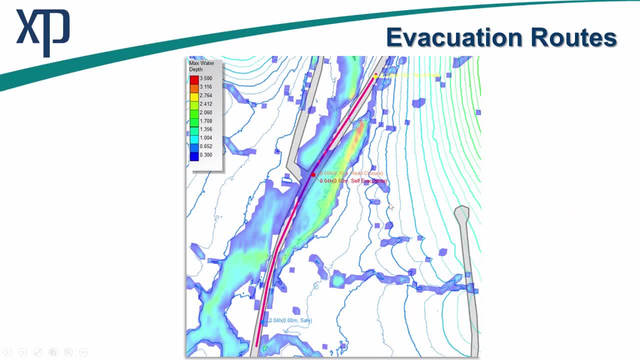 so how much time would the farmer have to basically move the sheep across the bund and get to the higher land? we can set up an evacuation route line along the bund, or in this case, it's showing along a highway how long until the water reaches a certain depth. 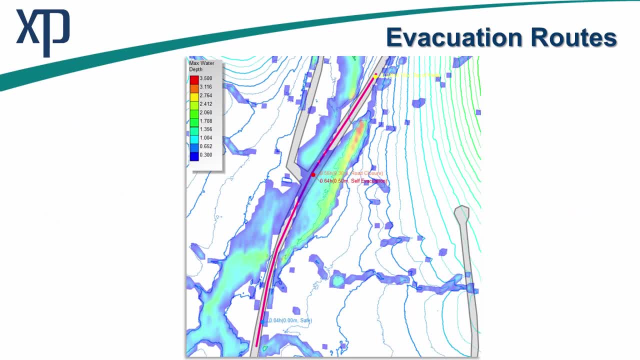 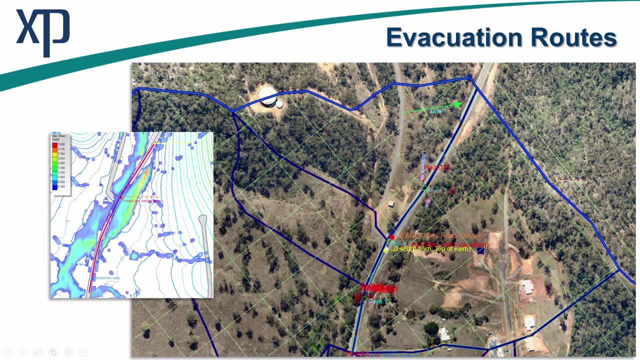 so it provides us with emergency plan information, which is very important. it's just showing you a background image of the highway and telling us that it will take 0.57 hours for the water level to reach 300mm in the highway. so at what point does the road? 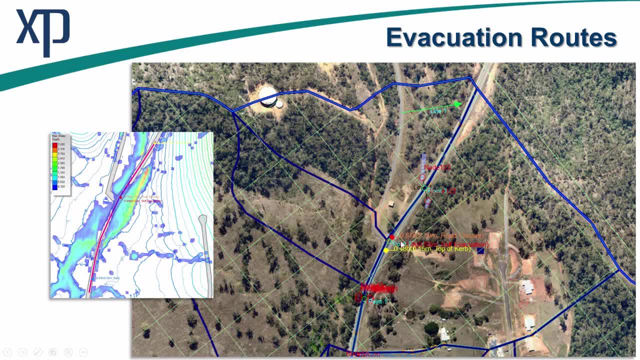 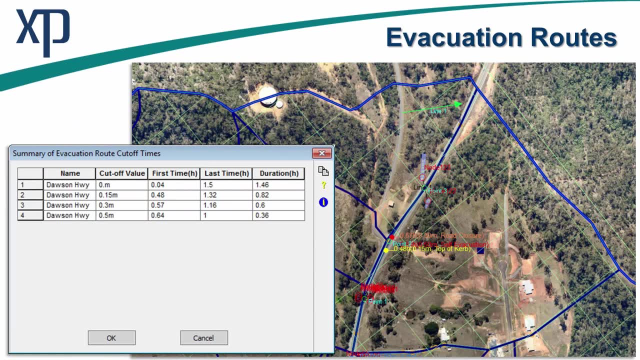 become impassable. it's after that period of time, so around about 35-36 minutes, in other words, of that event it's not just graphical output. we can extract from XP tables whatever information is contained within the programme, basically so you can set up the information. 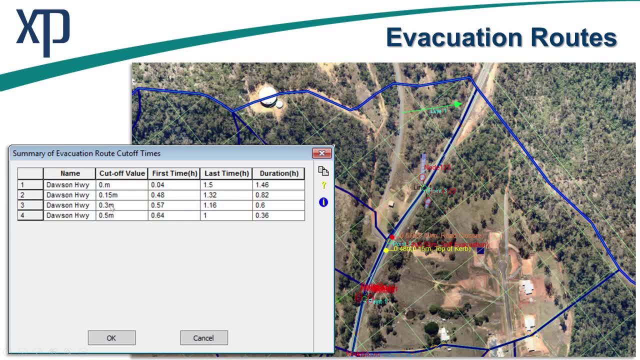 that you require to output, and in this case we've said: tell us how long until the water is reaching 150mm, 300mm and 500mm? how long does it take for that water to initially reach that depth? how long does that last for? so? what's the duration? 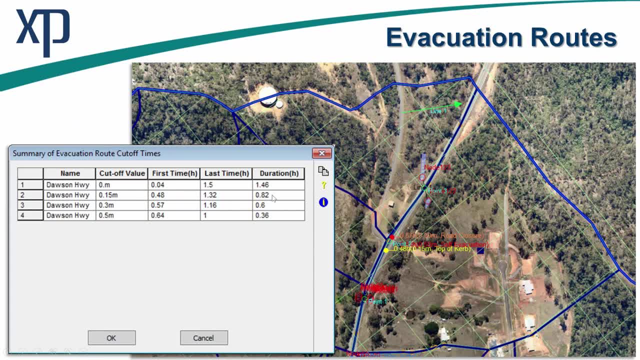 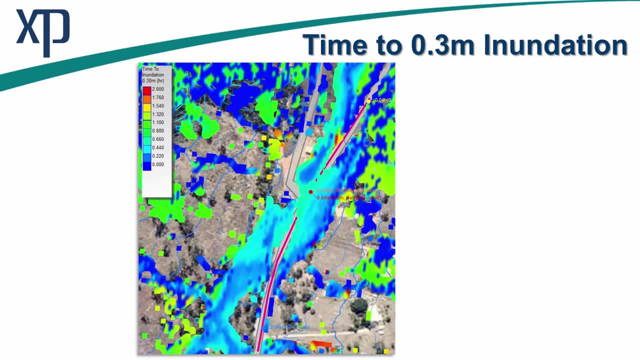 of time that the water is at that depth of 150mm or 300mm or 500mm, for example. this can also be illustrated graphically and we can extract this information in GIS format so that can come straight back into ARC if you want to identify properties. 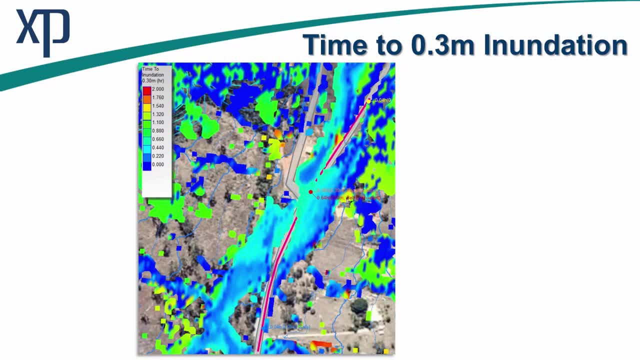 or buildings would be at risk for what period of time? so in this particular case, I'm saying: tell me how long this area will be under 300mm of water. so the light blue is telling me it's around about a half an hour when you get up to the yellow. 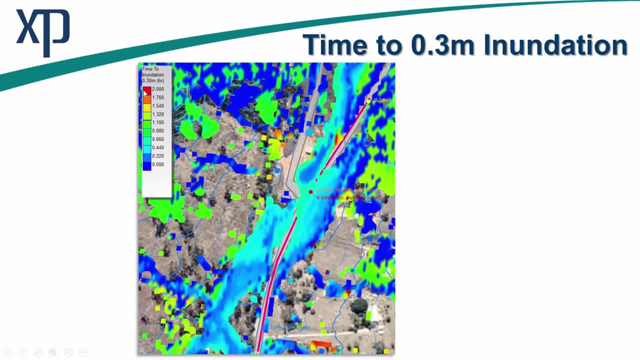 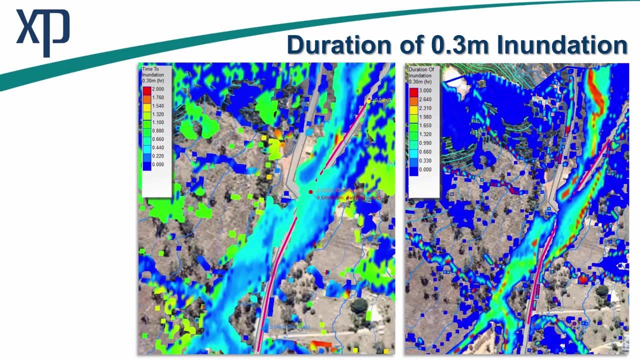 it's around about an hour and a half and when it's red it's two hours of inundation at 300mm depth helps you to understand the situation in the catchment. what's the duration of the inundation? so how long will this area be? 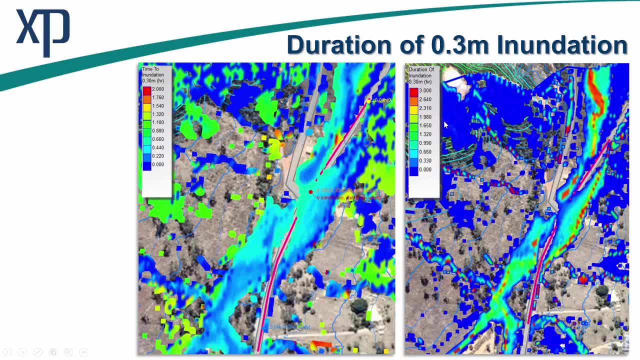 under 300mm of water. so the red is saying three hours. so this is the sort of channel section alongside the highway. here it'll be under 300mm of water for something in the region of three hours. the blue is a third of an hour, so 20 minutes, 15-20 minutes. 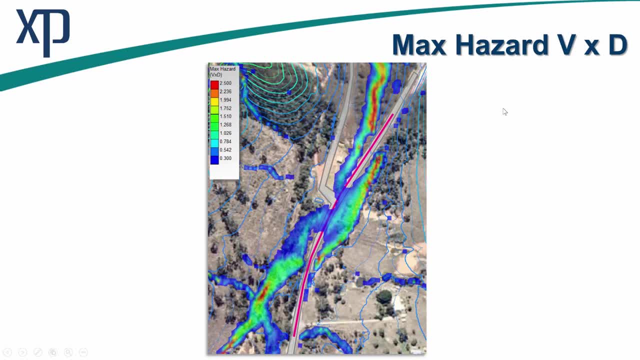 we can also combine this to look at the maximum hazard ratings. so, comparing the velocity of that water with the depth of the water to extract as the depth hazard rating requirements, and looking at the pure maximum depth of water that's occurred during any of the events, we can extract this information. 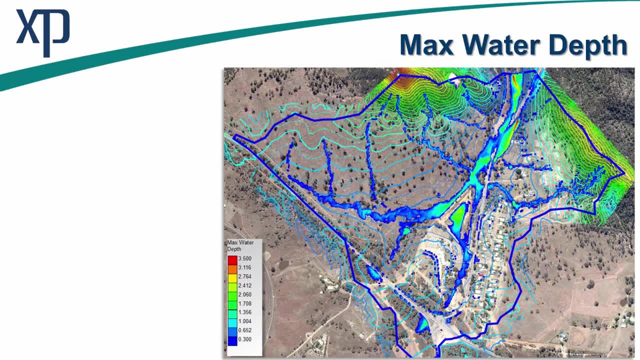 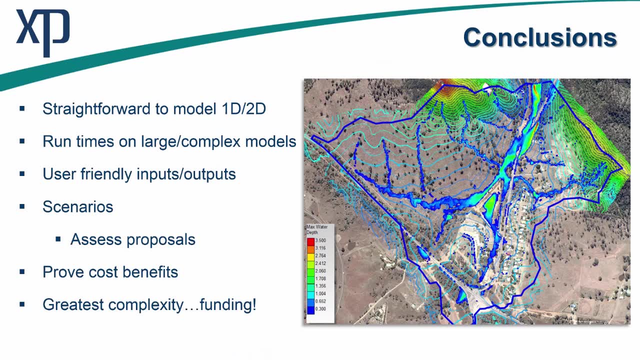 so, in conclusion, it's just relatively straightforward to model the 1D-2D combination. there is a little bit of work involved. rubbish in, rubbish out, I hear you all thinking, but with that information available it's relatively straightforward with a user friendly interface. 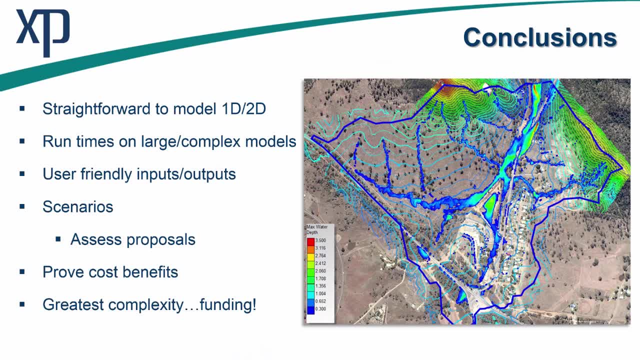 to generate this type of model. a word of warning on extreme large models. the run times will extend. so there are improvements constantly happening with all the software programs modeling to improve those run times for you. the 1D-2D combination will give you the best. 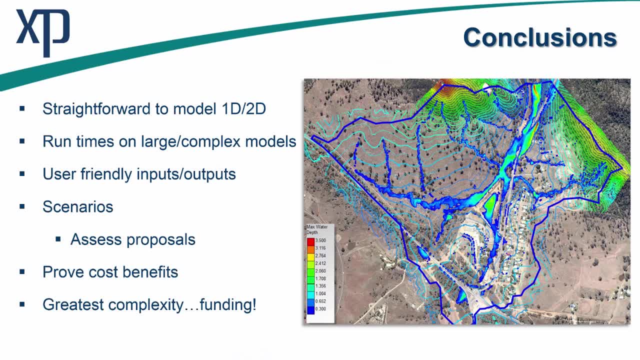 optimum way of working with this type of model. not only is it user friendly in terms of the inputs, but the outputs are extremely helpful. we could run videos of this as well, by the way, but output and take back into GIS would be the ideal way forward and we can run these various. 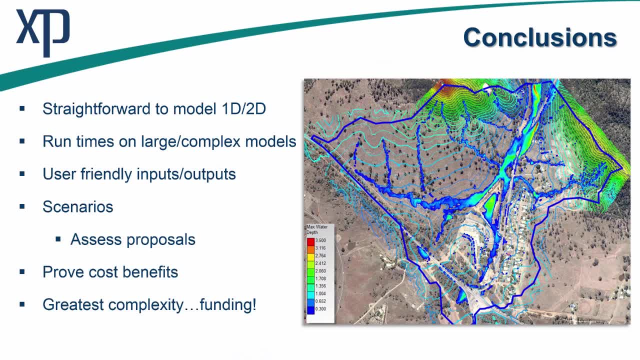 scenarios, to assess the proposals and put money to this, as well as explaining to the landowner, explaining to the farmer how long his crops would be inundated for, etc. so we can prove those cost benefits with the modeling. and moving on to the cost, the greatest complexity isn't so much the modeling, 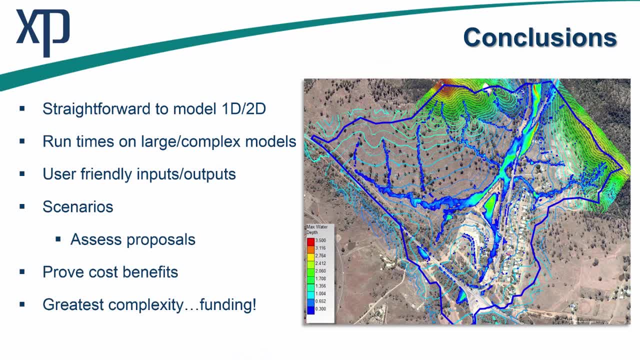 it's the actual funding mechanisms a lot of the reasons why these schemes won't go ahead. so any feedback. we will be running a short survey at the end of this, by the way, so any help with the funding ideas is one of the questions that Tom and I would be very interested to hear from you. 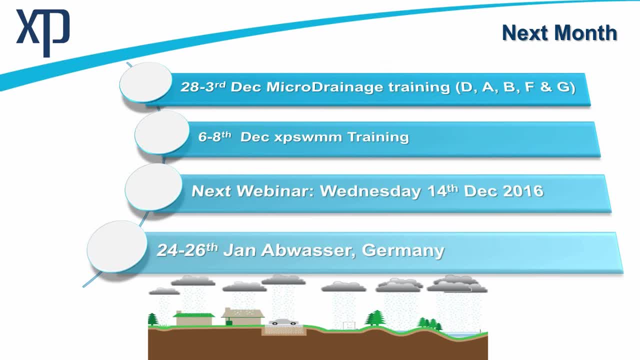 at the end of the presentation, so I hope that was of interest. I appreciate the questions that have come in before I go on to next month. there was one, Tom, that came in, where this caught my eye, but there are others that we will answer and send the answers back to everybody at the end of the 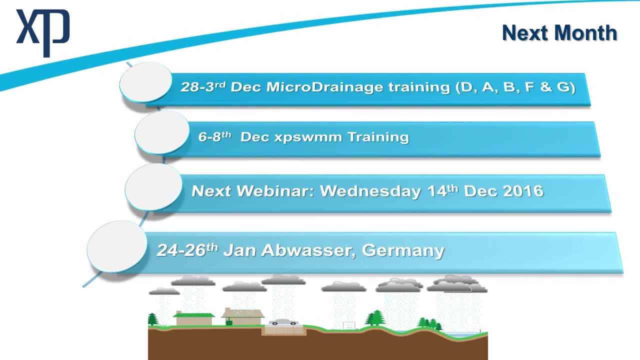 presentation. did you find any landowners that were able themselves to carry out the work, and were they competent especially carrying out that kind of work? it's an interesting question because actually most people assume that farmers and landowners all own tractors and 360 diggers and can do this sort of work. 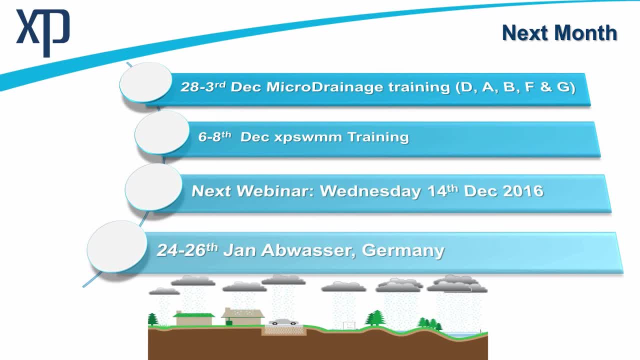 in practice. that's not always the case, so I would say most are across my particular study area, but there were times when we've had to consult with an external contractor. it's best to use someone local, someone that the landowner knows, that do the work and are proficient in this sort of 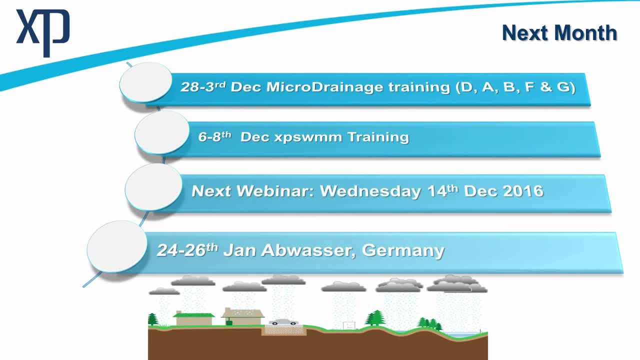 groundwork. thank you, and thank Tom for showing us the light at the end of the culvert. thanks for that. so, looking ahead to next month, folks, we have some training sessions coming up with XP Swim between the 6th and the 8th of December. I haven't checked with Marta. 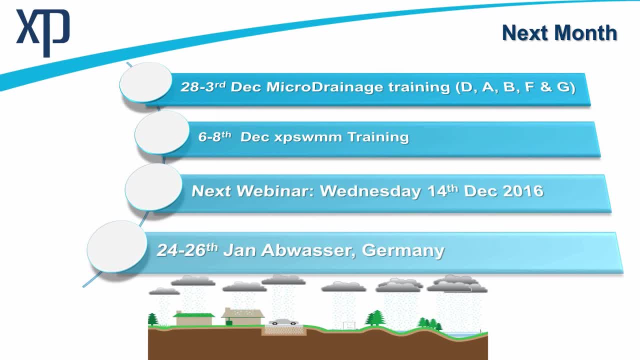 the numbers yet whether there are spaces available. I'm assuming that there are. just before that we're running a weeks training with micro drainage. it's really interesting for me because a lot of things that came out of Tom's study so far- the importance of local engagement. 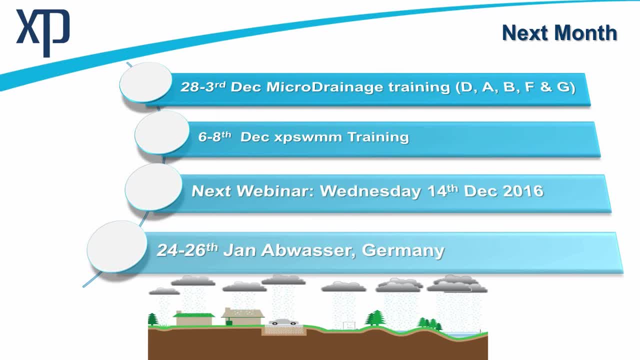 we don't underestimate local knowledge, the multiple benefits that are coming through from these schemes. there's very much a comparison with what we're doing at the local level on new developments with SUDS. I can see with the catchment scale with natural flood management techniques. 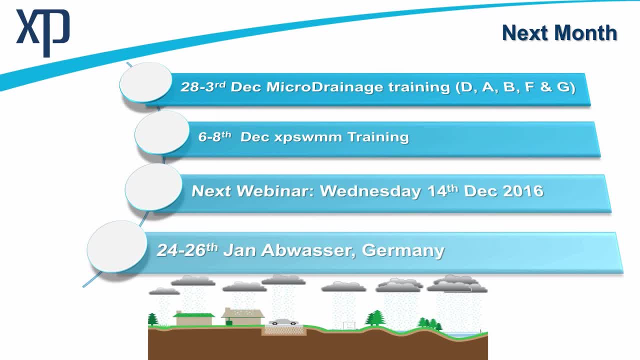 it's very interesting. the next webinar talking of what we're looking at next will be on micro drainage on Wednesday, the 14th of December. so you'll be more than welcome to engage with us and join us on that webinar. we'll send out an email so that you can register. 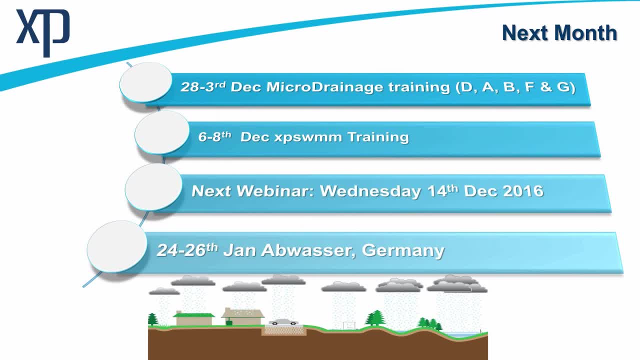 again. Stuart and the team will send out an e-cast to enable you to book for that, and Christian and the team. Christian Becker, our man in Germany, will be attending the Abwasser conference and exhibition over in Germany in January, so anyone listening in from Germany? 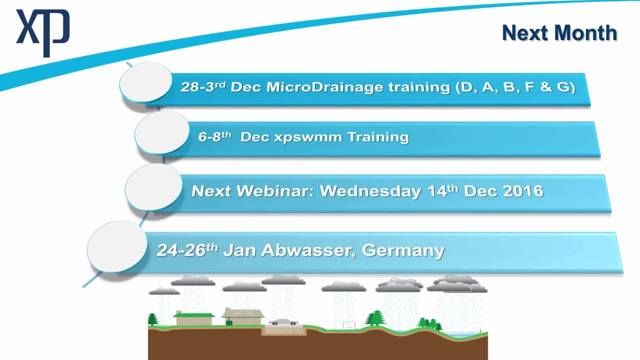 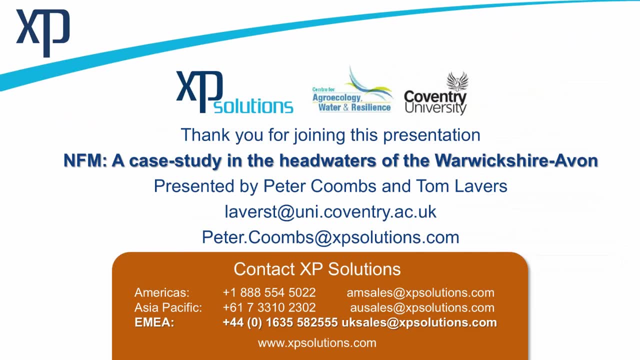 pop along and say hi to Christian and the team there. that would be great, Peter, we do have some questions which came in some of them. yeah, sure, we've got time for questions. I'm looking over my shoulder and I was a little bit anxious on the time. 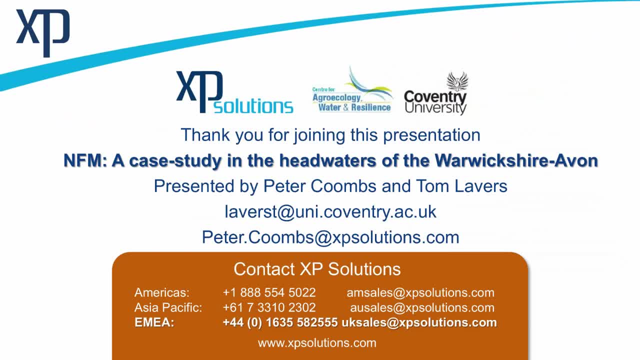 but that's great. if you want to go to the questions, I'll do this really quickly. we have a question from Simon. when decoupling flood peaks, have you been looking at adjoining possibility and different storm durations for the smaller sub-catchments to prove the intervention? 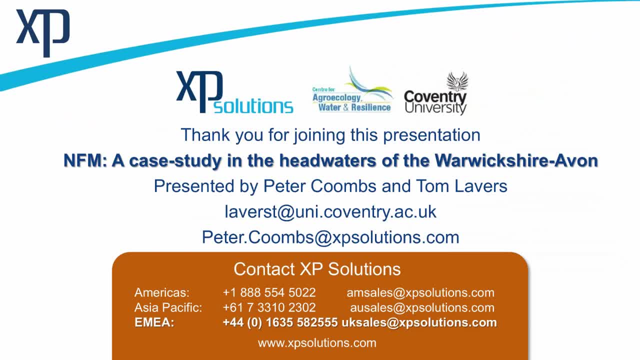 that makes the peak worse in all situations. yeah, that's a really valid point. so obviously, on this sort of scale, hopefully I made it clear earlier that you don't want to create an almost downburst effect where you are synchronising flood flows. so, as part of the scenario planning, 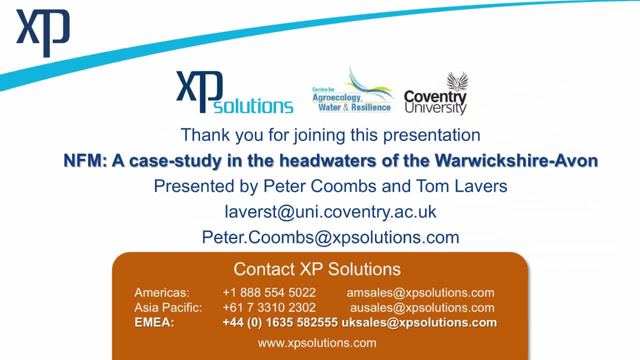 and understanding the temporal relation between all these different sub-catchments and flood propagation. the SWMM model will include separate hydrographs, as it were, for each of the delineations that can then ultimately augment the hydrograph to indicate basically: are we really attenuating the overall flow? 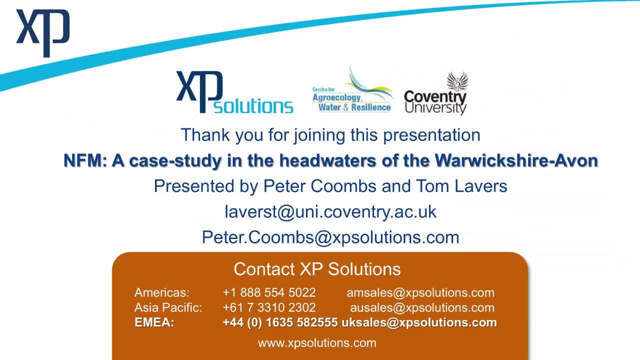 so that's a really valid question. there is another question from Cam: is there any initial findings of reduced flood risk to the downstream properties? isn't that the question? yes, well, principally on volumes, on a local scale, for example, the Cam, cumulatively that volume has been showed. 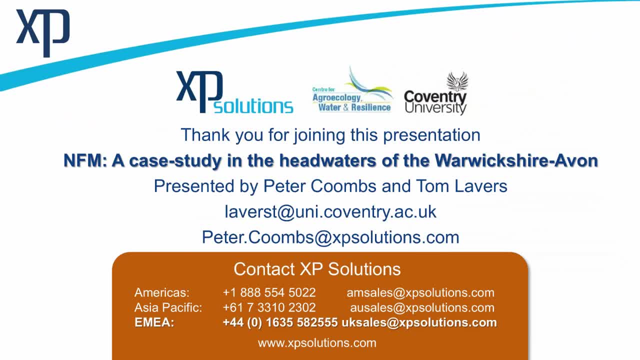 to slow the flow and lower the volumes that are entering Chipping Camden, which is the downstream settlement, but on the MISO scale, no. and for the same answer really as the previous question, that I really need to sort of hone in with my modelling: the influence of desynchronisation. 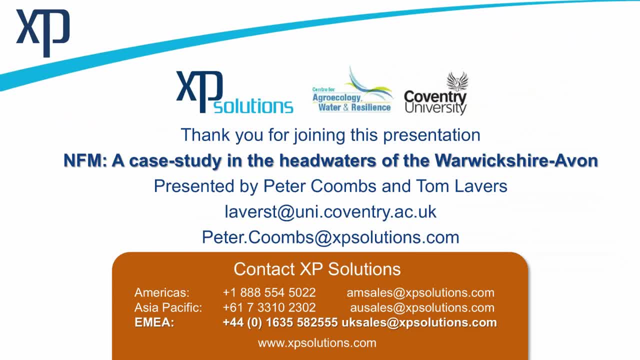 at lowering risk and obviously saving properties, as it were. so I hope that's partly answered. another question from Ray: how much calibration actually is involved. how much calibration have you done, or you can't yet answer how much. I hope to do some informal calibration with the sort of networks. 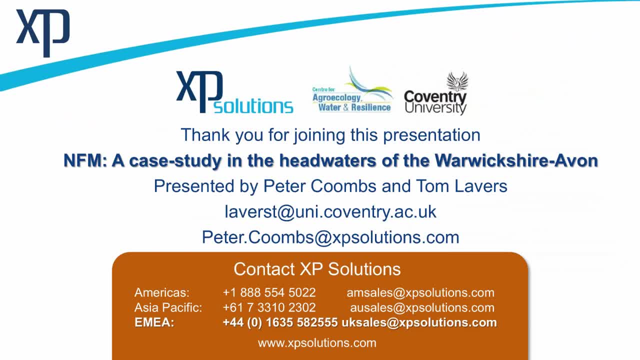 of farmers using existing images that they have across the catchment of particular events that then I can reference to as well as, interestingly, there are 4D sources for calibration as well. so some of the farms are private organisations that advertise on social media and over. 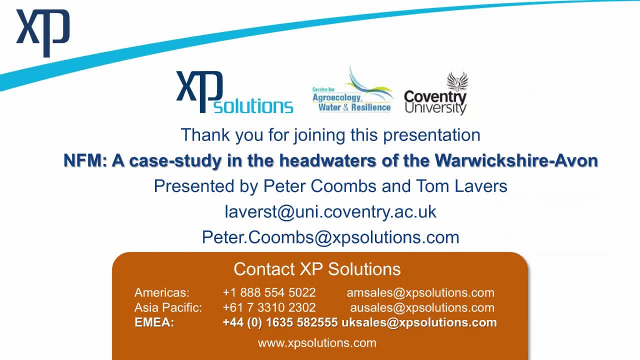 particular events. they have taken images of the event that I can then refer to on a sort of numerical scale as well. I have got some sort of triangulated rainfall data that I hope to do some sort of regression analysis to to identify, basically, the relation to the discharge data peak over thresholds. 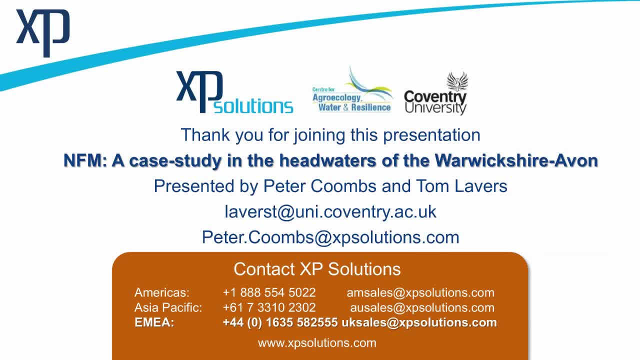 and an ultimate sort of hydrograph that can indicate how accurate the data was? Is it worth mentioning that there is the one gauge in the river, but it is the downstream. there is one major downstream gauge at Mitford Bridge, just south of Shipston on Stour. 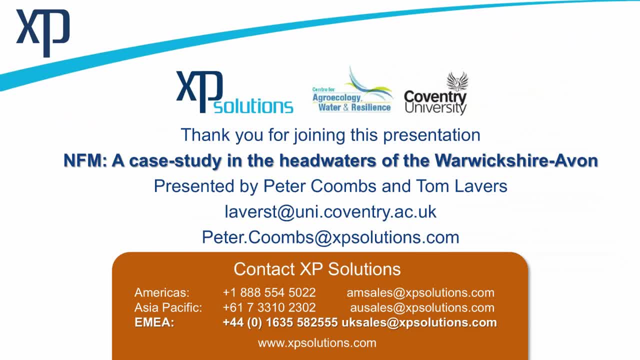 but it is in the Stour, isn't it? just downstream of the confluence of the three rivers, so we don't have anything up each of the catchments. Yes, so obviously calibrating each of the delineation contributions is there is less confluence because we are past.